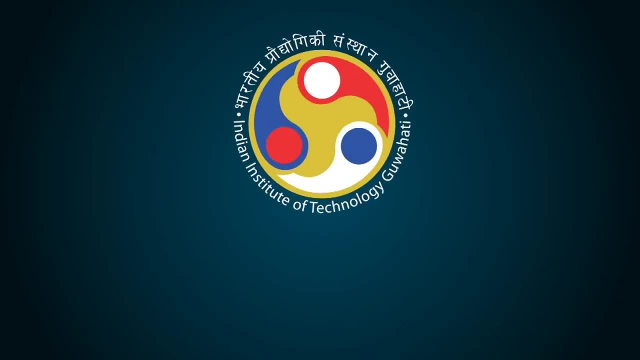 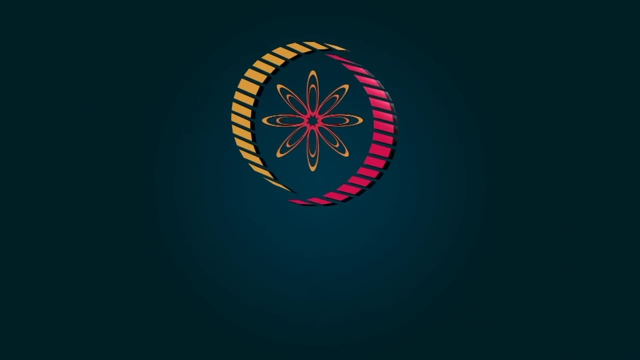 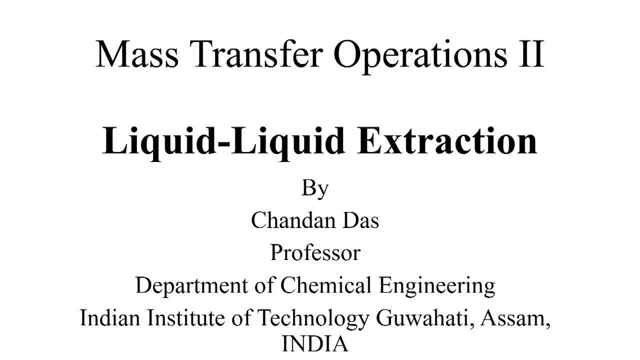 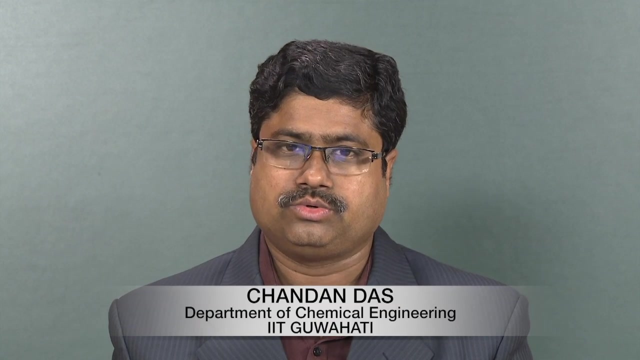 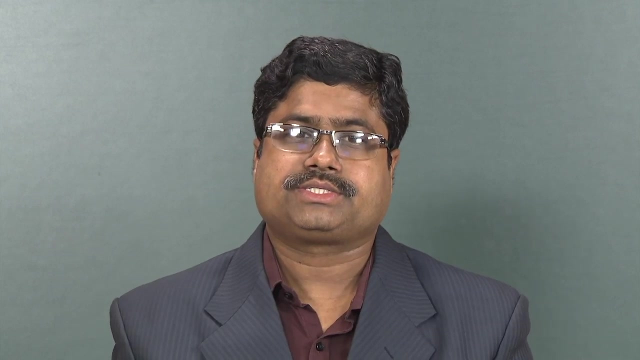 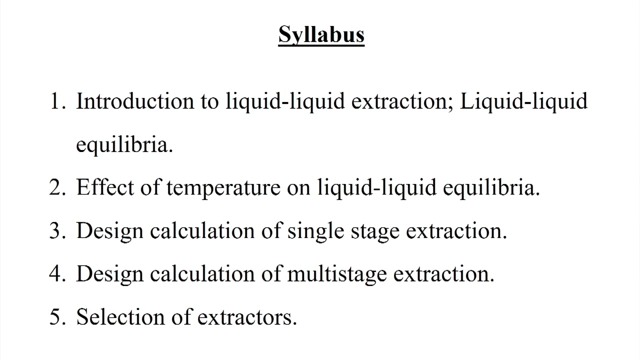 Welcome to mass transfer operation 2 course. Today I will start discussing on this liquid-liquid extraction. The syllabus is as follows: Introduction to liquid-liquid extraction, liquid-liquid equilibria, then effect of temperature on liquid-liquid equilibria: design calculation. 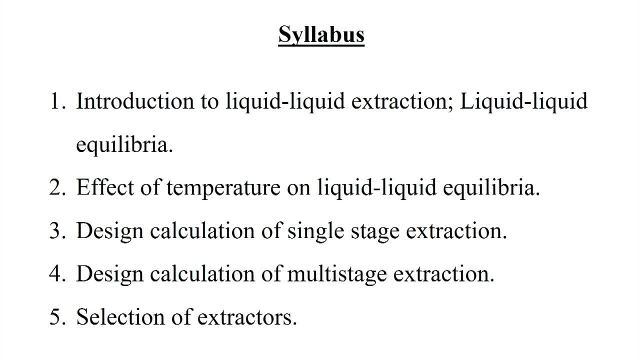 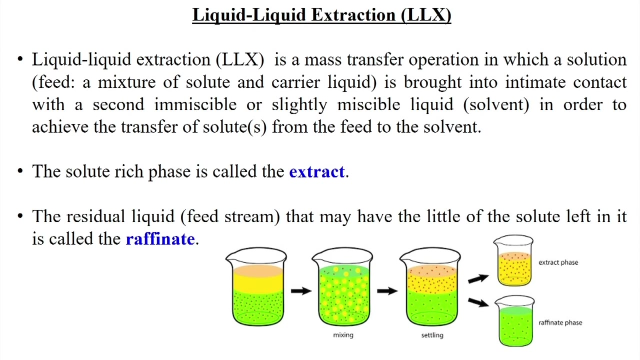 of single stage extraction, design, calculation of multistage extraction and, finally, selection of the extractors. Now we will be discussing on introduction to liquid-liquid extraction, followed by this liquid-liquid equilibria. So in the beginning we need to understand the process. liquid-liquid extraction, That is, liquid-liquid extraction- sometimes it is. 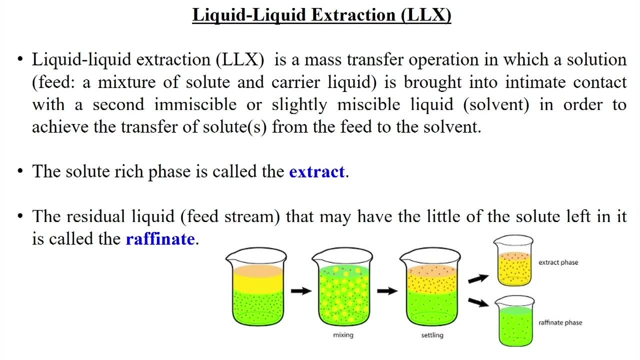 designated as LLX. It is a mass transfer operation in which a solution containing this feed, that is, a mixture of solute and carrier solid, is brought into intimate contact with a second immiscible or slightly miscible liquid in order to achieve the transfer of the solute. 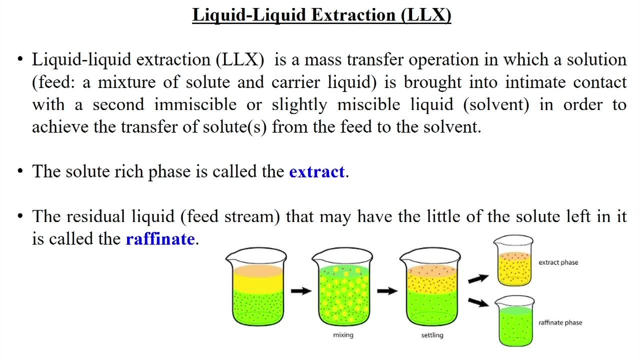 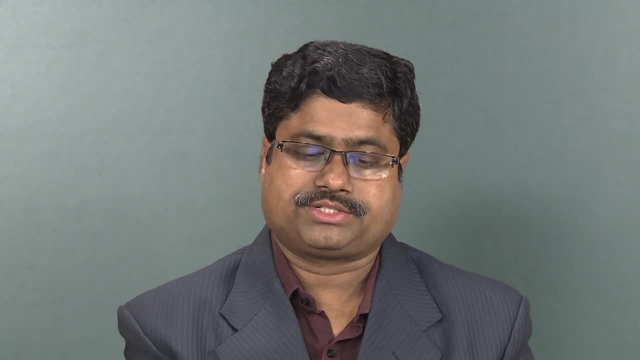 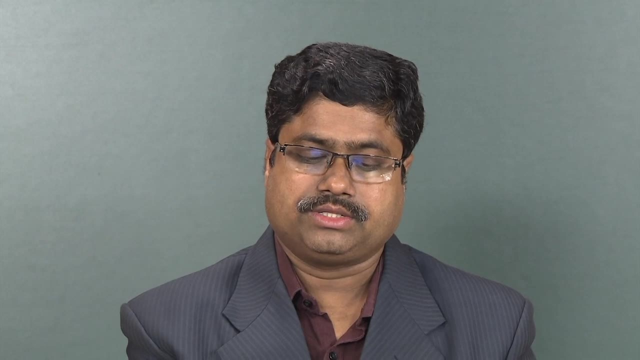 or solutes from the feed to the extracting solvent. The solute rich phase is called extract and the residual liquid that may have the little of the solute left in it is called raffinate. So if we say this one schematically, say the feed is of this dots, and with the we can say 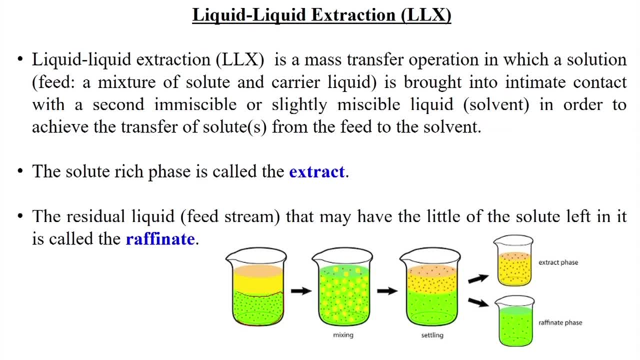 the carrier solvent. it is initially there in the beaker and then second liquid actually is fed inside this beaker and it is mixed properly to get this suppose, homogeneous mixture and it is allowed for a long period of time So that the two liquids will be separated. 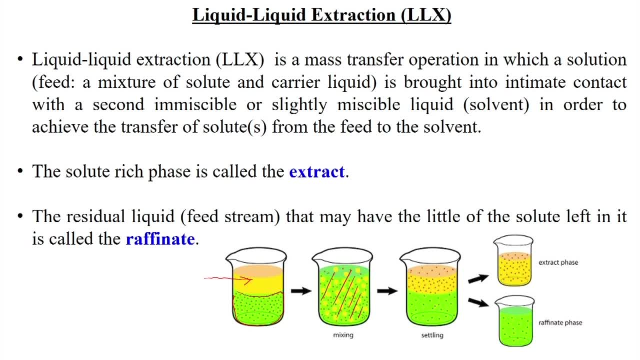 from each other due to this density difference and this solute- or this, we can say this- one target component, that is, the dot, now is distributed like this: it is maximum amount of the dot has gone to this extracting solvent and minimum amount of the solutes are present in the carrier. 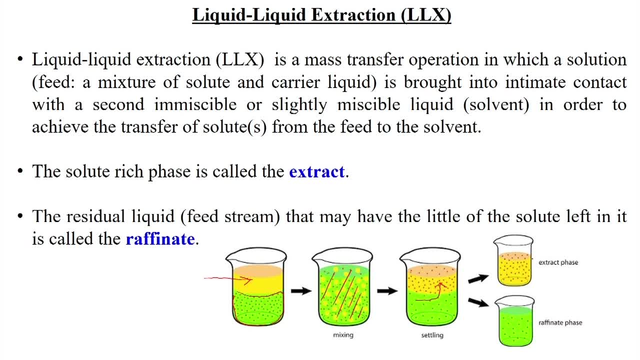 solvent and if it is allowed for a long period of time, then it will be separated into two different liquid phases. this one is that we can say this one rich in the solute, that is, we can say this one extract phase. and the raffinate means the exhaust phase, where the 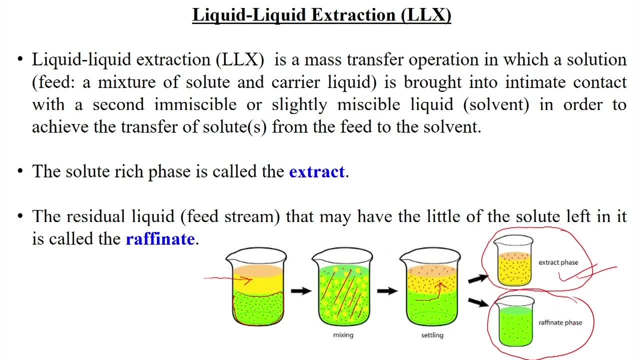 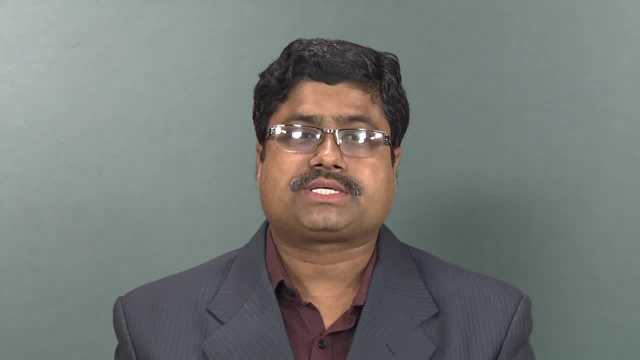 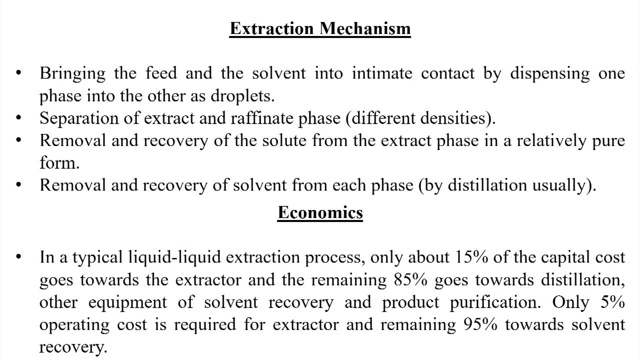 we can say, this small amount of the solute will be present. Now this extraction mechanism there is. this is very simple mechanism that firstly, we need to bring the feed and the extracting solvent into the intimate contact by dispensing one phase into the other, as the droplets suppose. in the beginning we have the feed with the 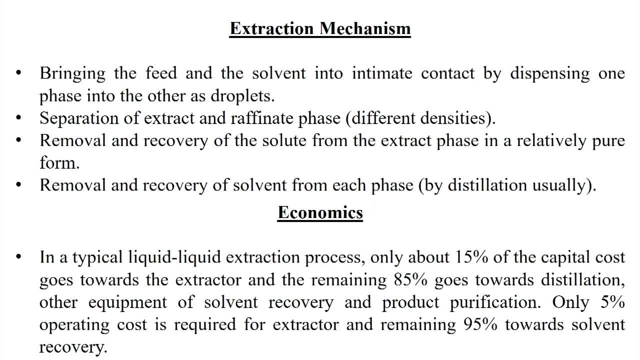 solute and the carrier solvent, and then we will be adding this extracting solvent into this feed and then you we have to mix this properly so that it will be dispersed as the droplets. Now, depending on the miscibility of the target component- that is solute in the extracting solvent, say, these two will be separated into. 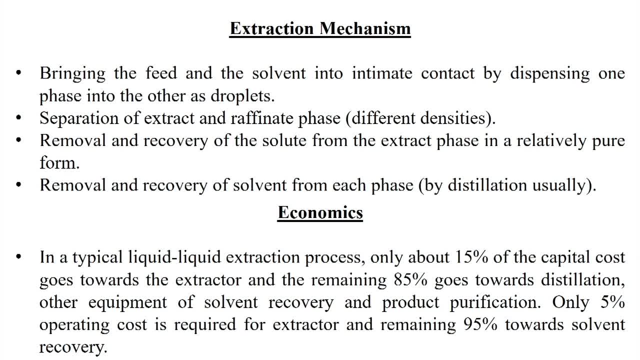 the two different, say the solute will be moving from this carrier solvent to the extracting solvent. so now we can say the second step will be separation of the extract and the raffinate phases. so it is dependent on the density difference between the two solvents. 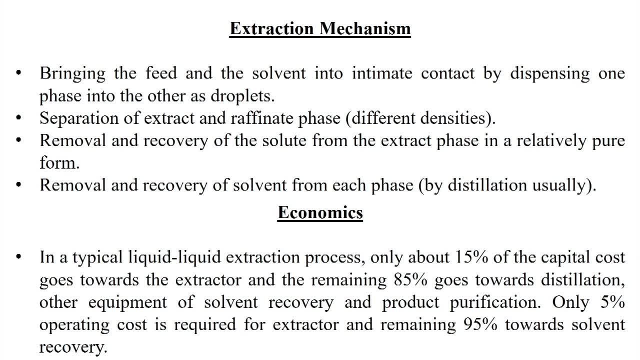 Now we need to do. the third step is that, a most important step, that is, removal and recovery of the solute from the extract phase in a relatively pure form. and the fourth one, that is- we can say this one- the residual part, that is, removal and recovery of the solvent from. 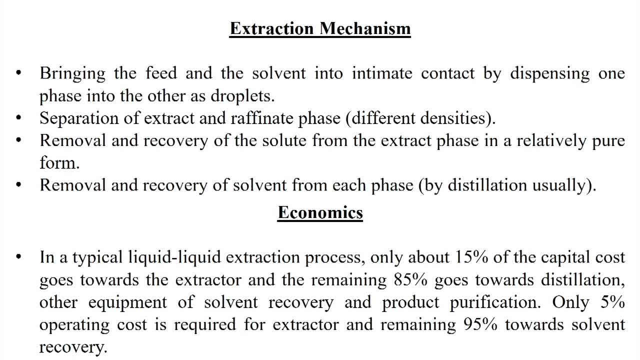 the say from each phases like this. we can say this one from the extract phase as well as this raffinate phase, so by distillation usually, but there are so many other ways also. Now if we talk about the economics of the extraction process, then it is very interesting. 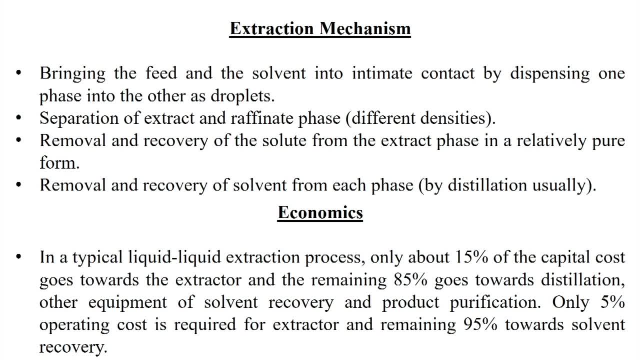 also, in a typical liquid-liquid extraction process, only about 15 percent of the capital cost goes towards the extractor and the remaining 85 percent goes towards the distillation, or we can say this: one other equipment of the solvent recovery and product purification and in terms of we can say this, one cost only 5 percent of the operating cost actually is. 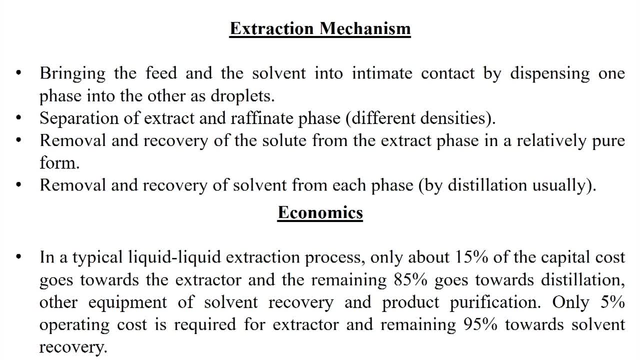 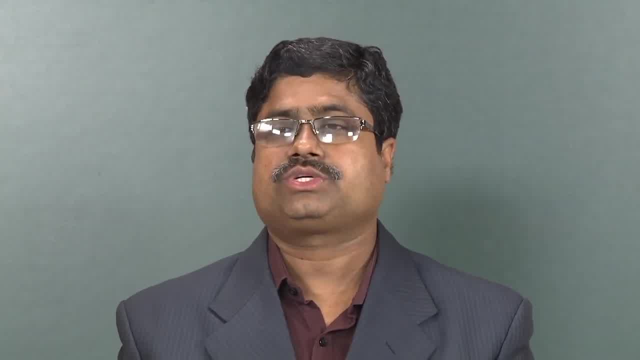 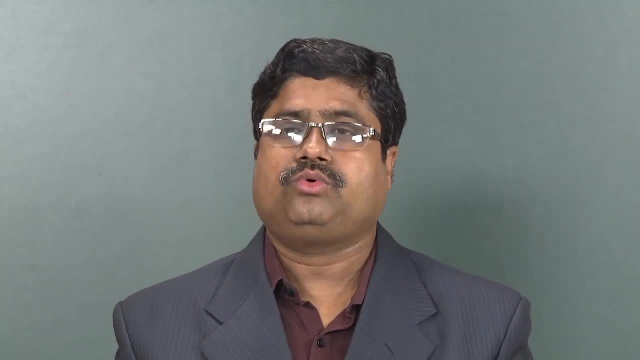 required for extractor and remaining 95 percent towards the solvent recovery. so we can say the from the economic point of view The extraction is not stand alone process but it is dependent on other separation process. but if there is no other alternative other than extraction we need to go for that. 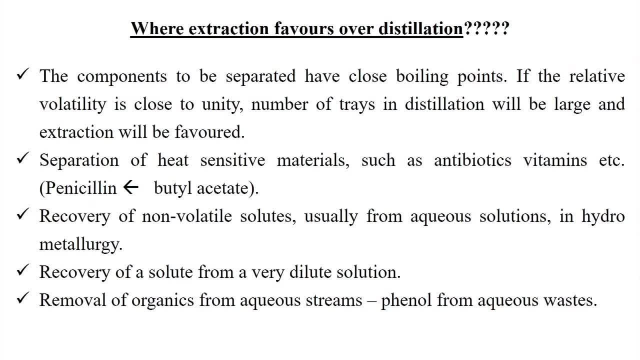 So we will be discussing this one, like where the extraction favours our distillation process. so there are so many, but here we are giving some examples like this: the components to be separated, So we have this close boiling points, then distillation, using distillation. we cannot 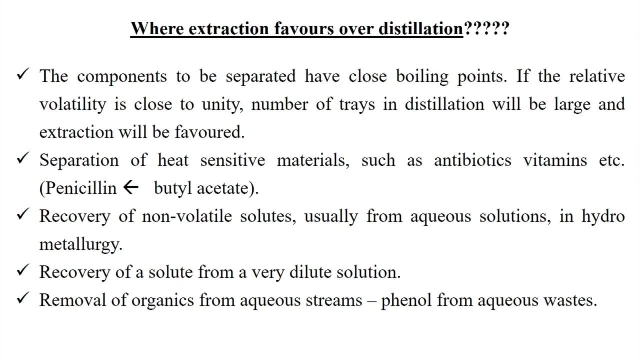 be separating these two components. if the relative volatilities also are close to unity, then number of trays in the distillation column will be very large and then extraction will favour over this distillation process. sometimes we can say this: one heat sensitive material to be separated, like antibiotics, vitamins, etcetera, using this extraction process. 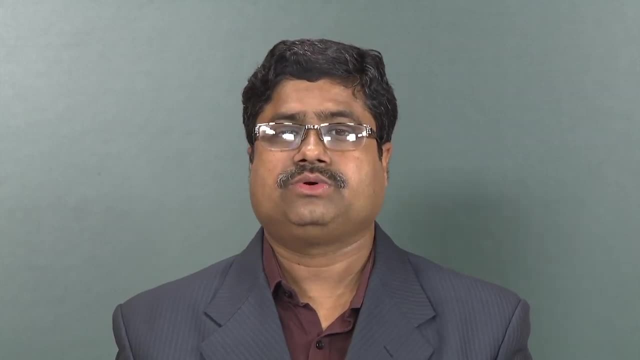 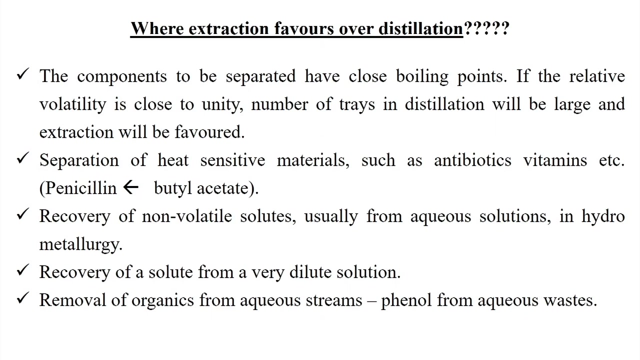 then we can say this: one heat sensitive material to be separated, like antibiotics, vitamins, etcetera. Then we can say distillation process, Sometimes the recovery of nonvolatile solute, usually from aqueous solutions in a hydro medicines. that is done by extraction process and suppose therefore very dilute solution there. we cannot. 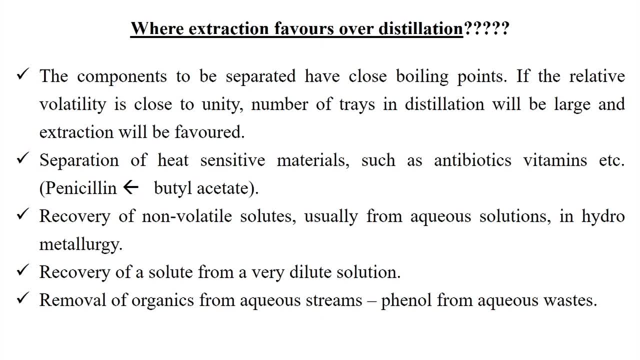 separate using this distillation process or any other processes, but there extraction process can efficiently separate the target components from the dilute solution. ози of the organics from the aqueous streams, like phenols from aqueous wastes, are done by extraction process where that cannot be separated by distillation process. 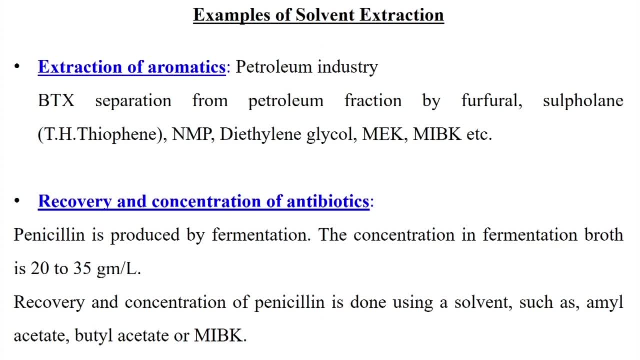 So few examples of the solvent extraction process we will be discussing here. then we will be going into the details of the extraction process, like this. first example is extraction of aromatics in petrochemical industry, like this: benzene, toluene, xylene. these are separated. 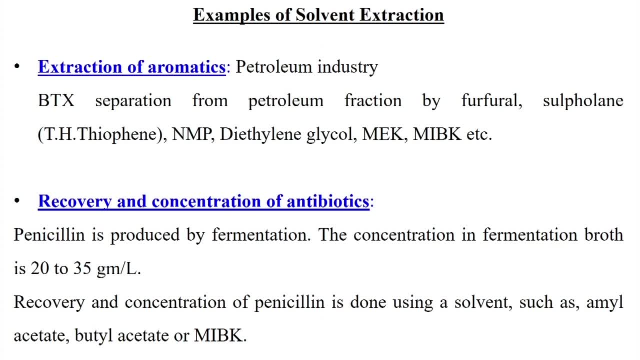 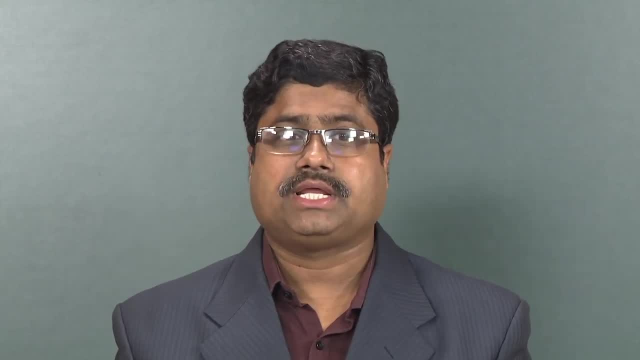 from petroleum fraction by furfural sulfolane or NMP diethylene glycol or methyl ethyl ketone or methyl isobutyl ketone, etc. these are all extracting solvents And recovery and concentration of antibiotics like we can say penicillin, it is only recovered. 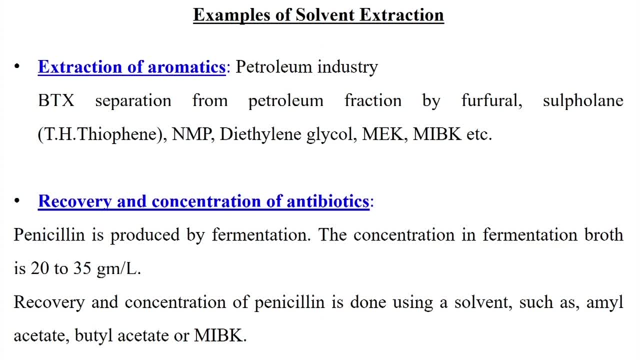 using this extraction process. Like the penicillin is produced by fermentation- we know this one from the fermentation broth- we can separate this penicillin using this extraction process. The concentration of the penicillin in the fermentation broth ranges from 20 to 30 gram. 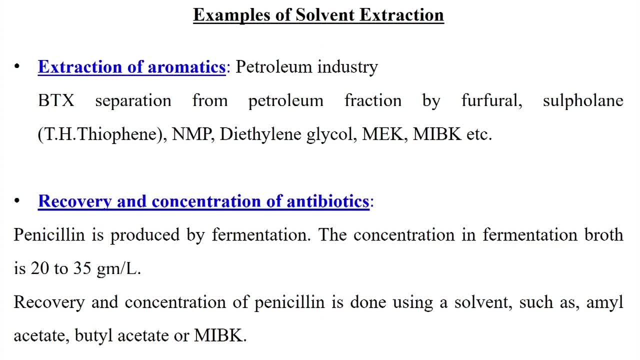 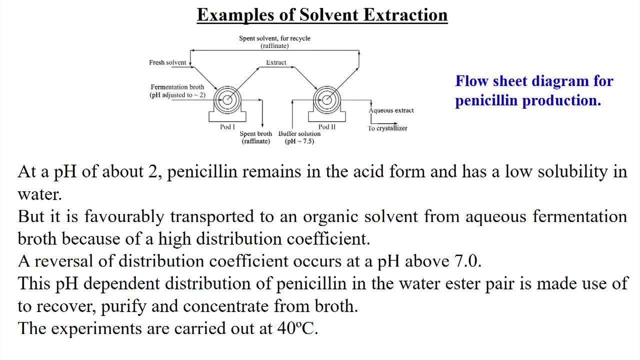 per litre and the recovery and concentration of penicillin actually is done usually using a solvent such as, say, amyl acetate or butyl acetate or methyl isobutyl ketone. So this is the process. We can get this one very schematically. we can explain this one very easily like this: 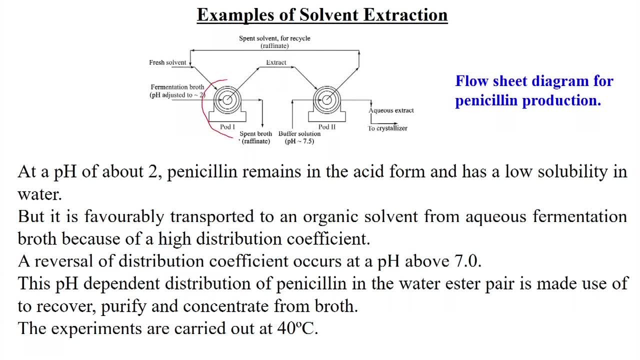 so we have this fermentation broth like this: around pH 2. it is extracted using in the water. So we can say this: at around pH 2. penicillin remains in the acid form and has a low solubility in water, but it is extracted in this system. but once we will be increasing the pH up to 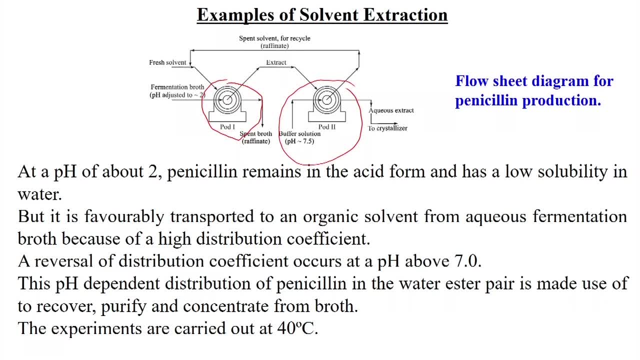 7.5. So what it favourably transforms. So this is the process. It is transported to the organic solvent from the aqueous fermentation broth because of the high distribution of the coefficient. So whenever we will be adding some amount of the solvent here and then say we can say 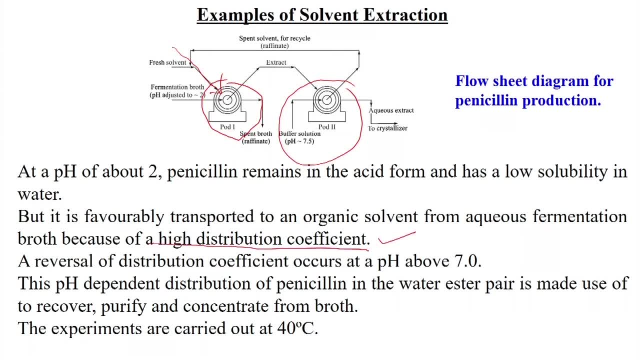 this one. due to this high distribution coefficient it will be going to this organic solvent. Then this one pH is maintained at around, say, 7.5. so in that pH- say this pH actually dependent. distribution of penicillin in the water restoration. In the water restore pair is made use of to recover, purify and the concentrate from the 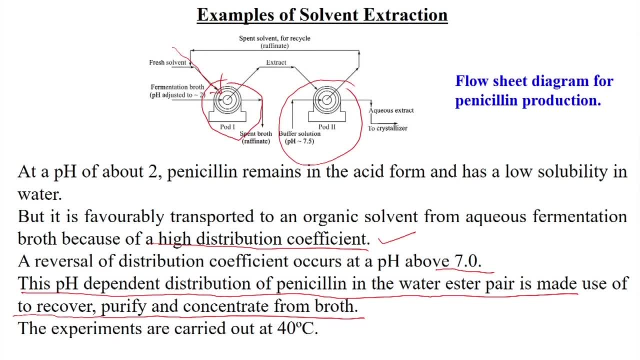 broth. Total experiment actually is carried out at 40 degree Celsius, So at pH 7.5 it is. we can say this one. the penicillin actually comes to the aqueous extract and whatever the solvent actually is used here to extract, it is now almost free from. 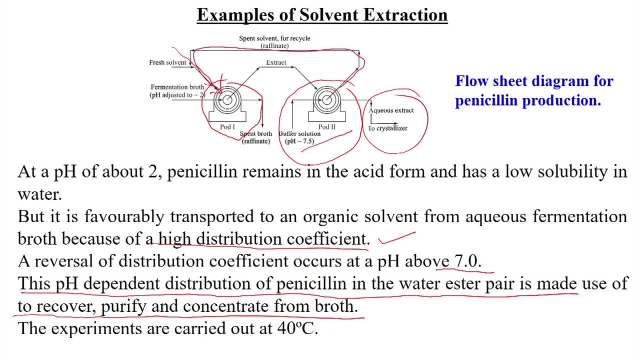 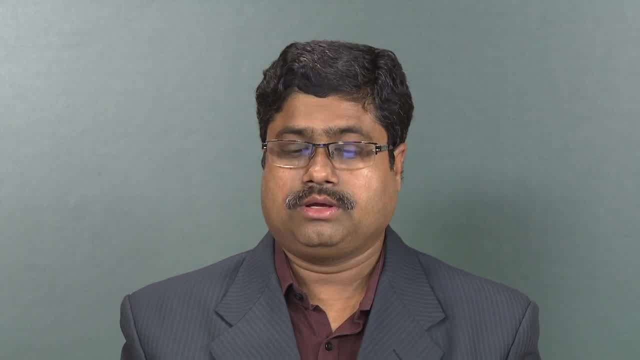 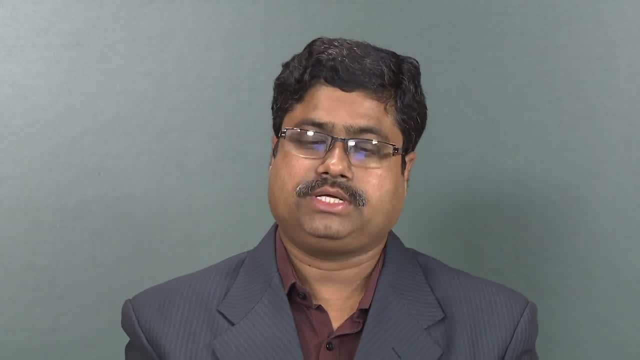 the penicillin, it is recycled back to the system. So this way we can say: this is the process, Thank you. So we can say this one, the extract, and we can say this one from the extract: after separating the target component, the, whatever the extracting solvent is again reused for the same extraction. 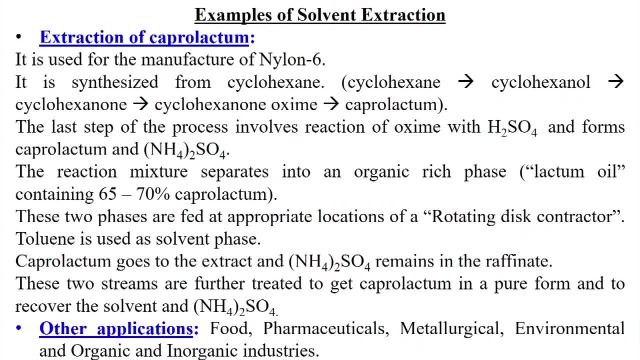 process for so many cycles. Now, the another example is the extraction of caprolactam, that is- we can say this- used to manufacture this nylon 6. So it is synthesized from the cyclohexane. We know this one. we are not going to the details of the process, but we will be discussing. 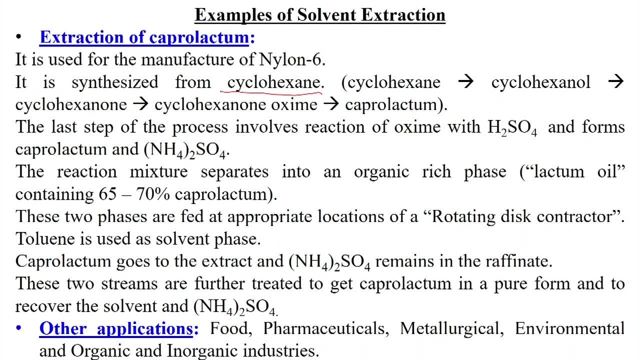 the one step where the we can say this one, we can use the extraction process to separate a particular target component, like this: cyclohexanone oxime, Like this: say: we can start with the cyclohexane, then from the cyclohexane to cyclohexanol. 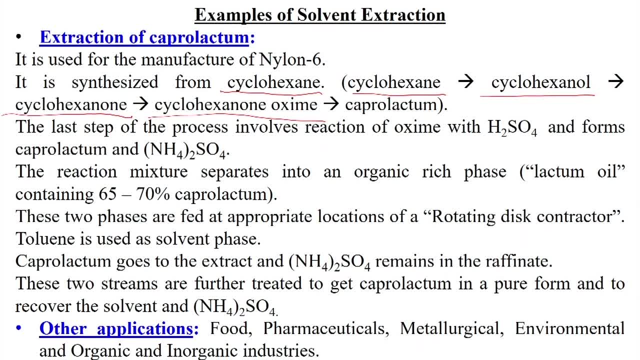 from then it is to cyclohexanone, then the step is cyclohexanone- oxime and then from the cyclohexanone oxime to cyclohexanone. Okay, So we can say this one is the extraction of caprolactam. 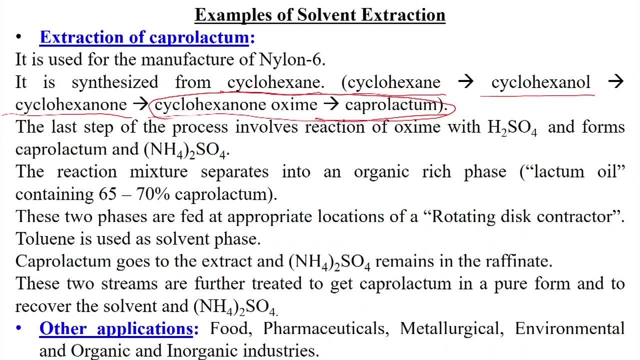 So in this step we can say this is the last step of the process- involves the reaction of the oxime with sulphuric acid to get the caprolactam and forms this caprolactam and ammonium sulphate. So the reaction mixture separates into an organic rich phase where we can say this one: 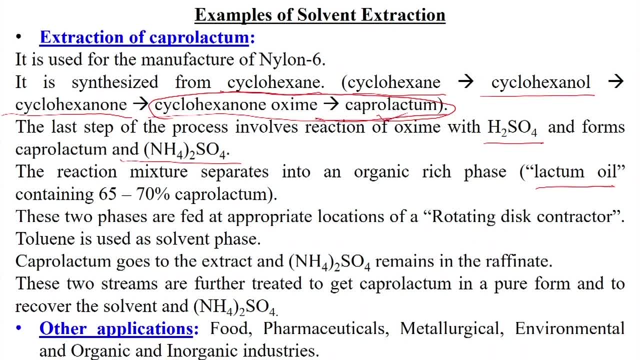 caprolactam is there that is called lactam oil. that contains 65 to 70 percent caprolactam. These two phases are fed at the appropriate locations of a rotating discontractor, that is, we can say this, one extractor. So this is the extracting unit, that toluene is used as the extracting solvent. 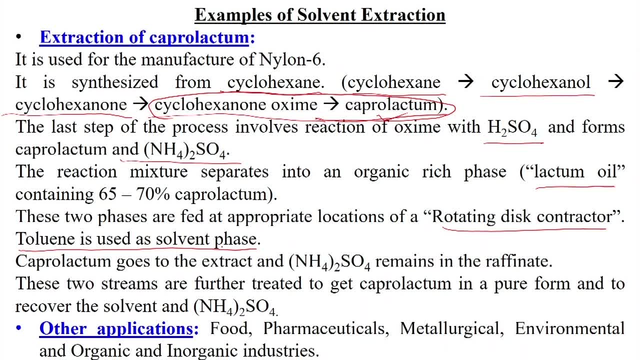 Then caprolactam goes to the extract means, say in the toluene phase, and ammonium sulphate actually remains in the raffinate or which is in the aqueous phase. These two streams are further treated to get the caprolactam in a pure form and to recover. 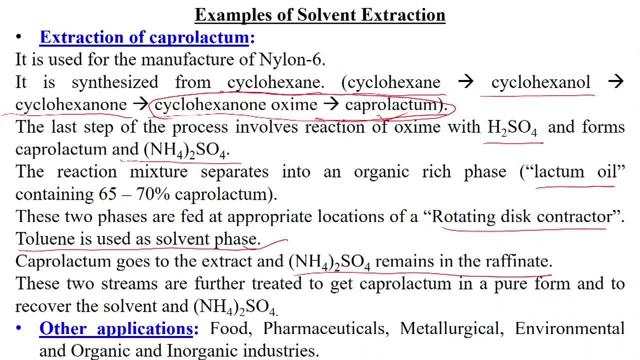 the solvent and ammonium sulphate. so all this will be again used for different purposes. Okay, Okay, Okay. So we have seen the extraction process like in food industries and pharmaceuticals, in metallurgical and say environmental and organic, and in running industry. 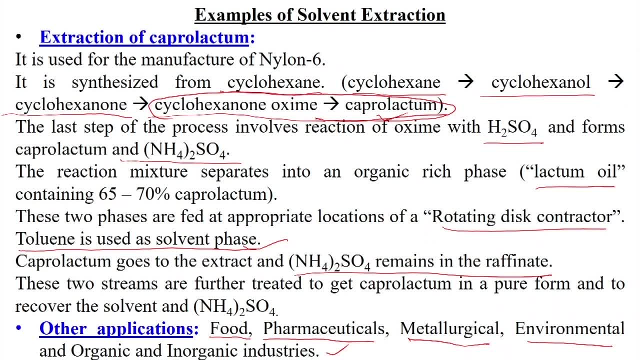 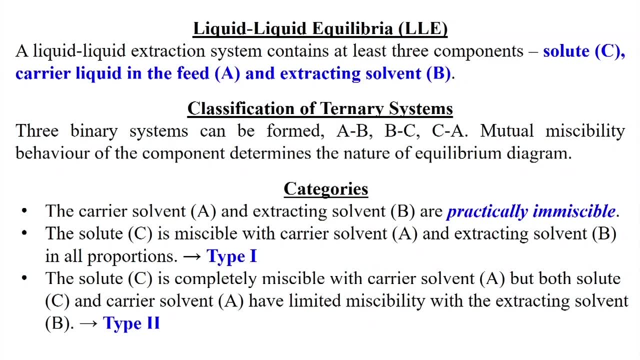 So there are so many applications of the extraction process. we will be discussing the details of the extraction process now. So before that, actually we need to understand the equilibria, that is, liquid-liquid equilibria, and now also we will be learning about the ternary diagram to understand the liquid-liquid 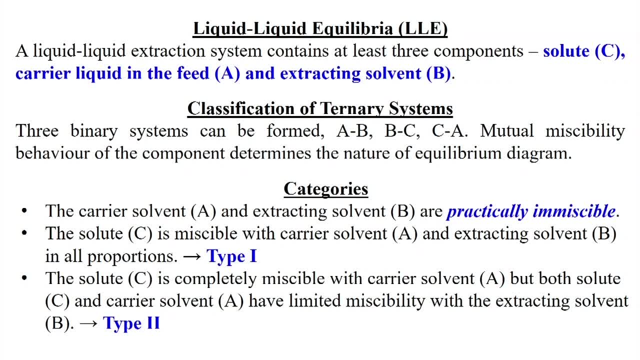 equilibria. Suppose our liquid-liquid extraction system contains at least three components like this, one will be the solute, that is, we can say, this target component. So we will take this as solute C and carrier liquid actually in the feed, that is, we can. 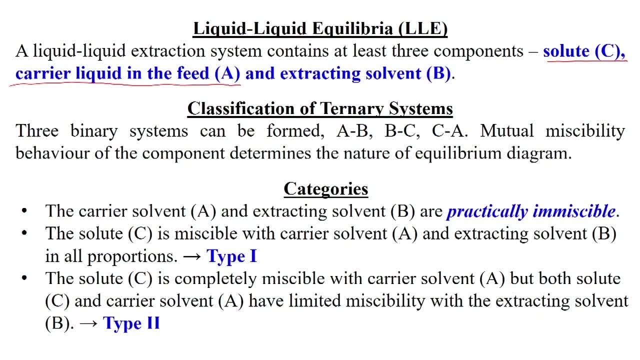 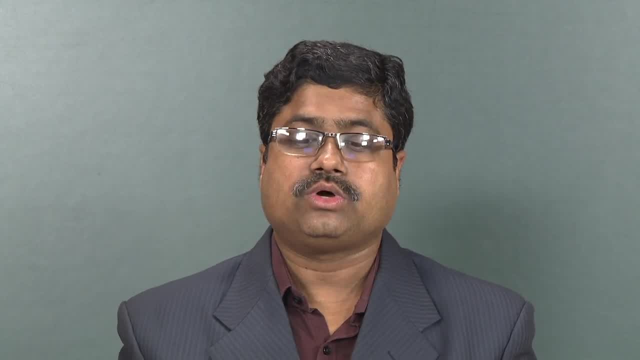 say this one when we have this feed, C is dissolved in A and we are adding this, extracting solvent from the outside. So this is we can say this one B For the entire extraction calculation, as well as this one whenever we will be discussing about the leaching process, that is say, solid-liquid extraction. 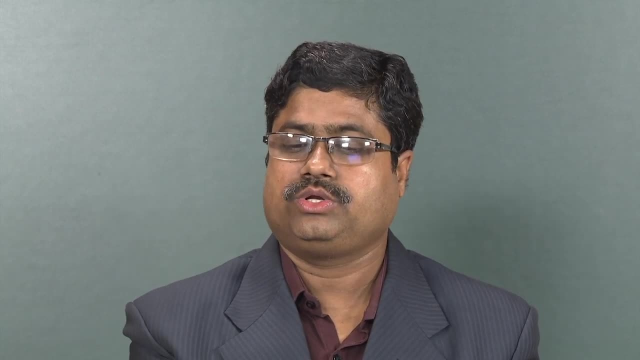 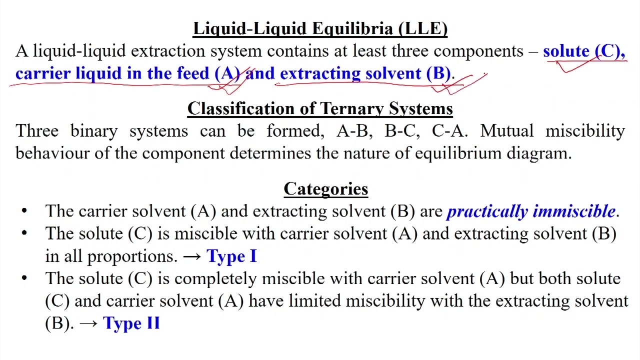 there. also we will be using these notations like solute as C, carrier liquid as A and extracting solvent as B. So now we need to understand the classification of the ternary system. Suppose now we have this A, this we can say carrier solvent, B is the extracting solvent. 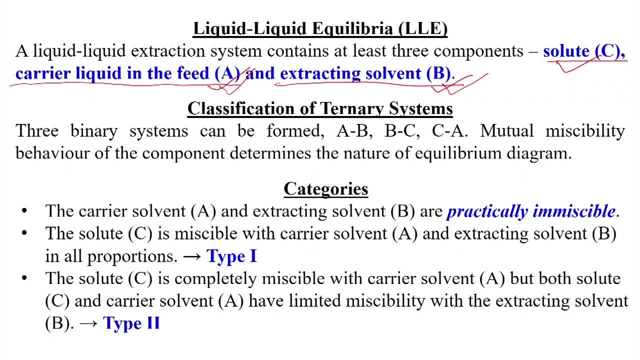 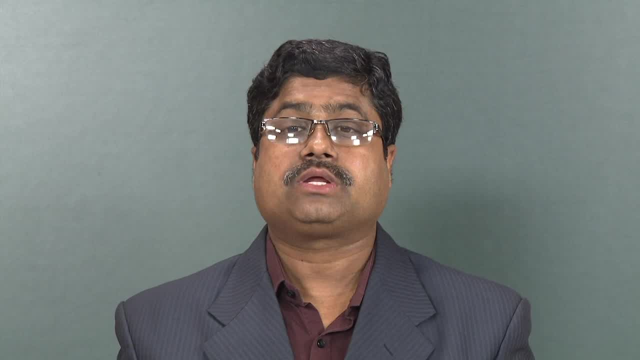 B is the solute. So out of these three components we have two binary systems like this, three binary systems: A, B, B, C and C A. So mutual miscibility, behaviour of the component determines the nature of the equilibrium diagram. 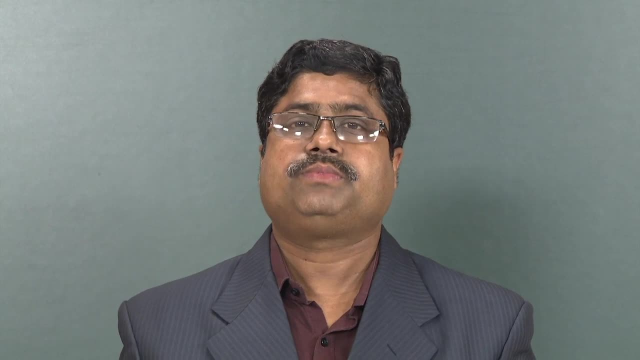 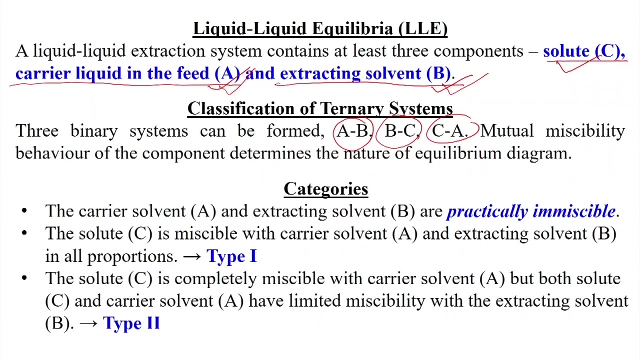 So what type of equilibrium diagram actually will be there that will be determined by the mutual miscibility of A, B and C, Like, say: the first system is the liquid-liquid extraction is like this, we can say this: one solvent and extracting solvent, say carrier solvent, and 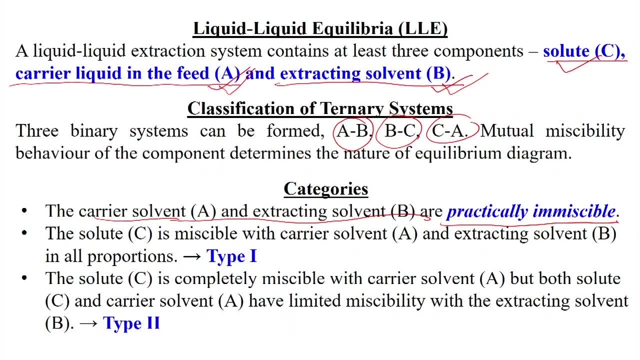 extracting solvent are practically miscible, immiscible. So that is, we can say this one, that is one system say we can say it is of no use in general. we can say this one: in the liquid-liquid extraction system, If solute is not, we can say this one miscible, this one. 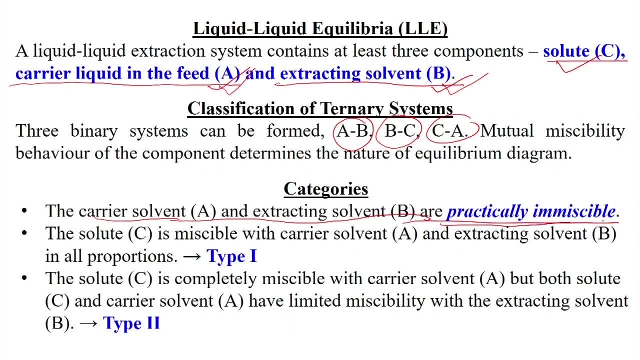 carrier solvent and extracting solvent are practically immiscible. So that is, we can say this one. these two are not miscible to each other, but we can say this one: solute C can be miscible with both A and B and the second type is called. we can say this one. 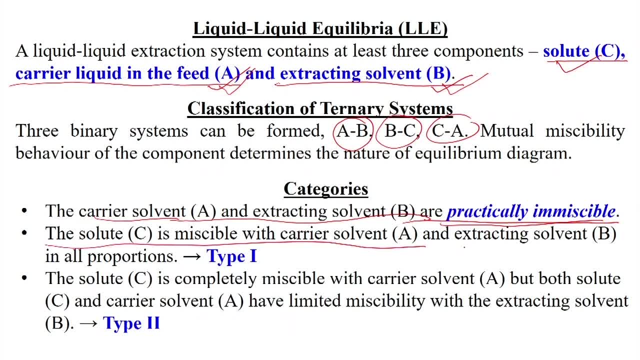 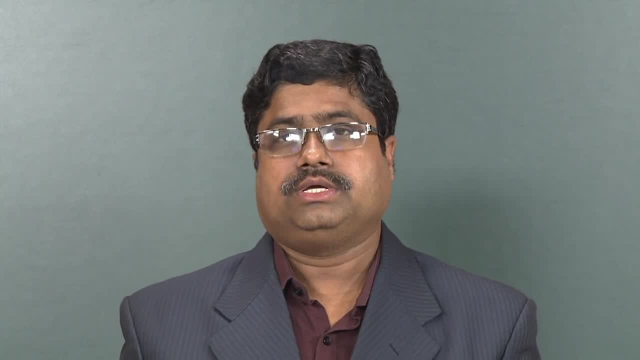 the solute is miscible with carrier solvent and extracting solvent in all proportions, that is, we can say this one type 1.. This is the we can say this one very good type of the solute. We can say this one ternary system where we can say this one, both carrier solvent and 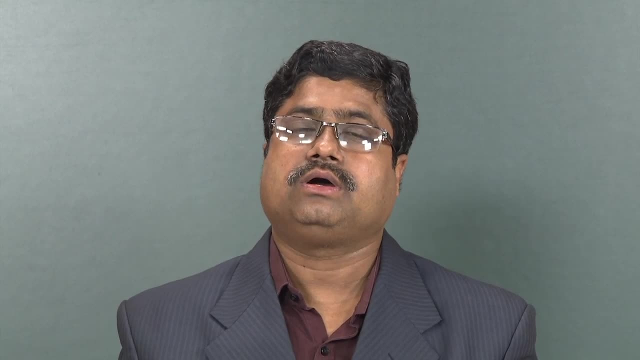 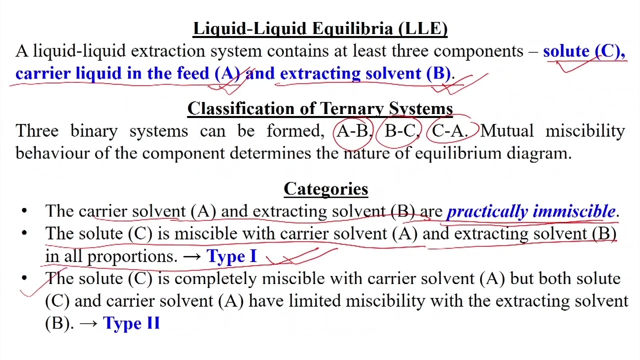 extracting solvent have the miscibility of target component in all proportions. and the last category, like this, we can say this one solute C is completely miscible with carrier solvent, where the feed is but both solute and we can say this, carrier solvent have limited miscibility with the extracting solvent B. So that is, we can say this one type 2.. So 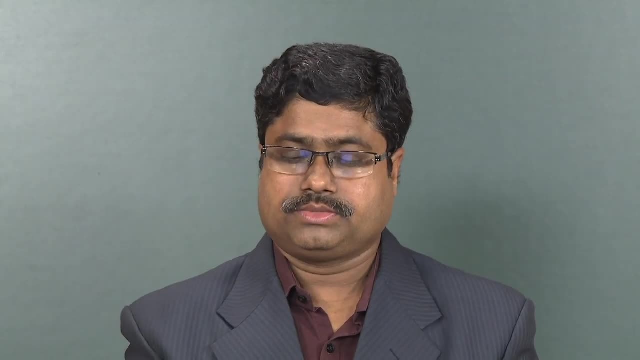 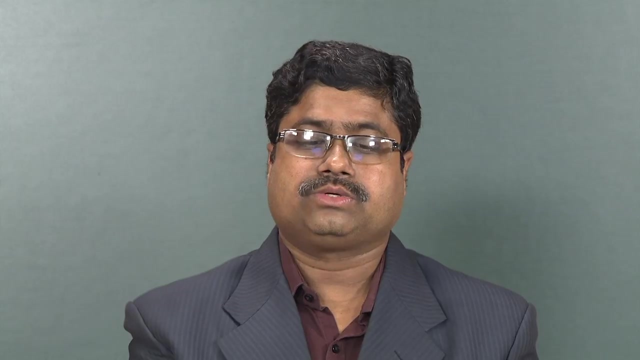 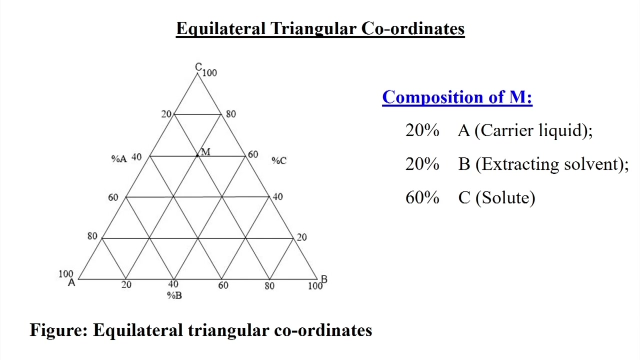 we have this, both type A1 and type 2, and based on their miscibility, actually we will be discussing the liquid-liquid equilibrium curve. So before that, we need to understand that equilateral triangular coordinate and we need to understand this very precisely, otherwise we will not be able to solve any extraction. 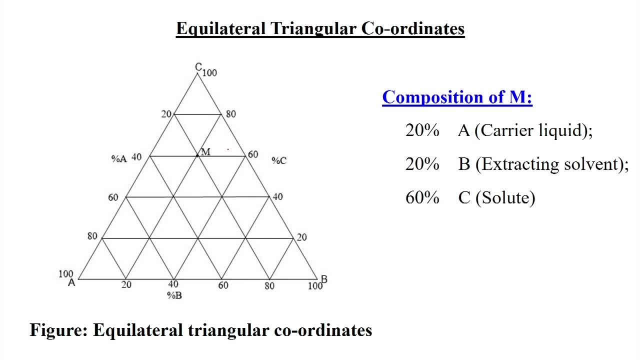 problem. So let us take a mixture of M, like here. So whenever we will be talking about say 100 percent A means this one, then say 0 percent A will be in this line. So this is. we can say 0 percent A, So this is 20 percent A, then this is 40 percent A, this is 60 percent A. 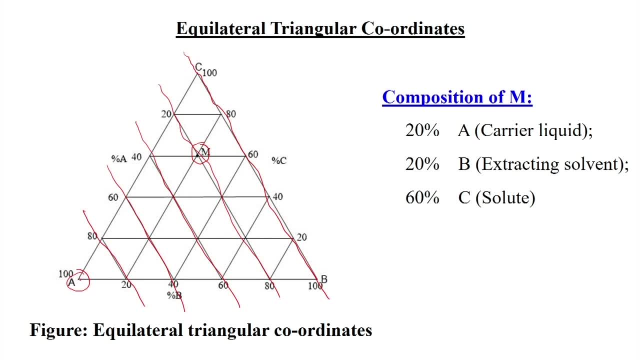 this line stands for 80 percent A and this tip is 100 percent A, So we can say this: for M, we have this 20 percent A, So we can say this: one carrier liquid, So this is the carrier liquid, contains 20 percent A here. So whenever we will be talking about this 100 percent, 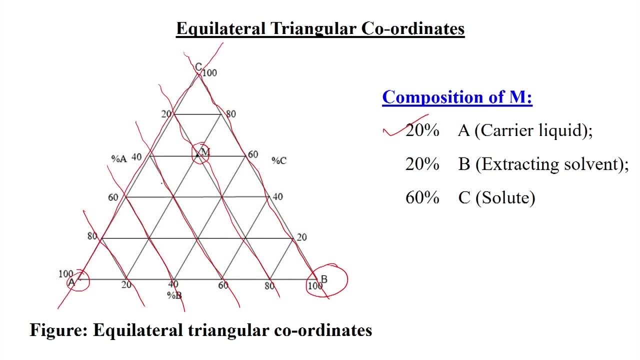 B means say this one. we can say this one: 0 percent B, then 20 percent B, then we can say 40 percent B, this is 60 percent B, this is 80 percent B, this is 100 percent. So this is. we can say this one: 20 percent B is there. So this one, Whenever we will be talking about. 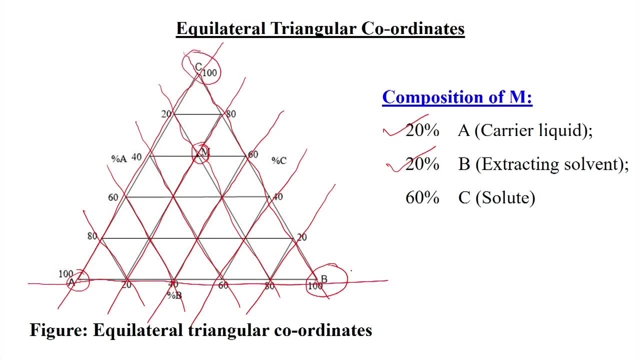 this: 100 percent C. So this is 0 percent C, this 20 percent B, then it is 40 percent B, So this one, we can say this one 20 percent B is there, So this one, Whenever we will be talking about this. 100 percent C. So this is 0 percent C, this 20 percent B, then it is. 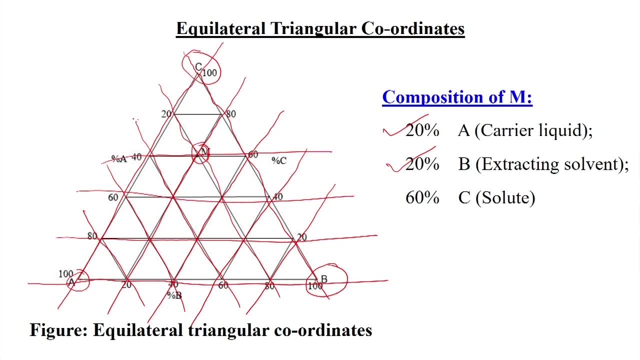 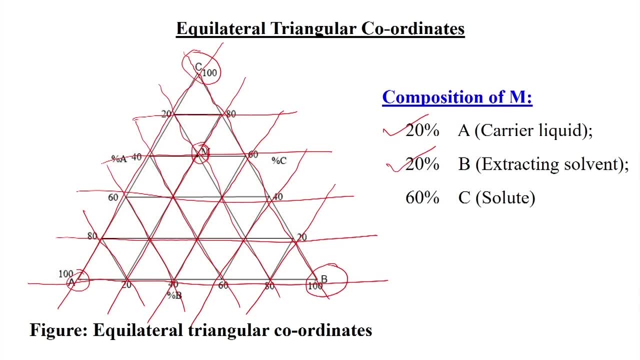 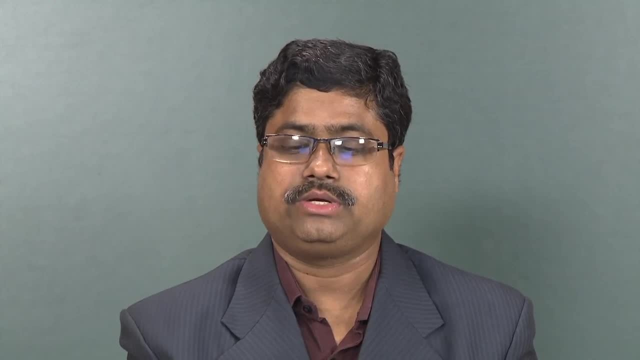 100 percent C. So this line, this one, corresponds to 60 percent C. So in all points C population is 60 percent. So then we can say this one for M, a contribution of A is 20 percent, B is 40 percent, 20 percent and C is 60 percent. So all these are actually in the liquid phase. 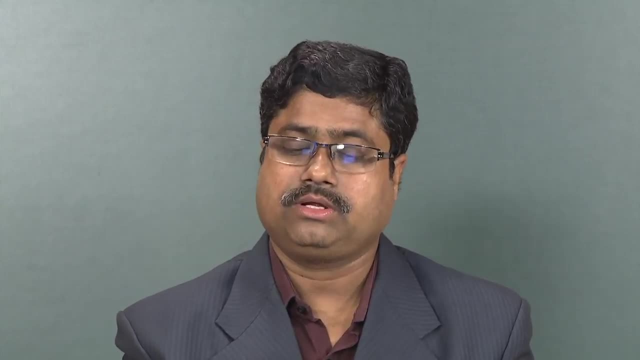 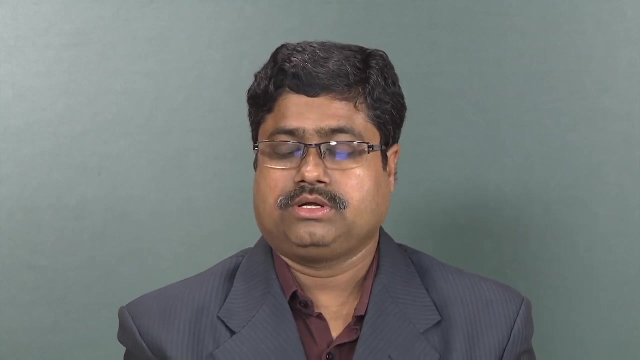 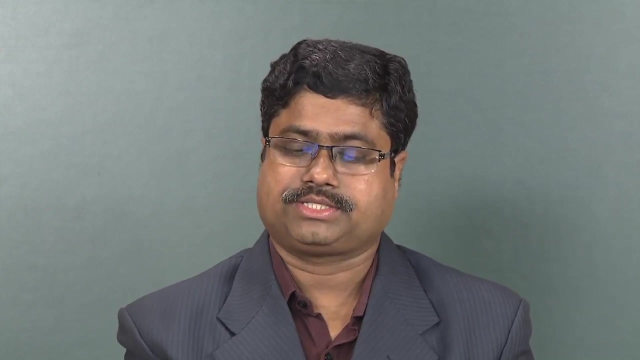 So all- A, B, C, all are in the liquid phase. So we can say this: one carrier liquid contribution is 20 percent, extracting solvent is 20 percent and this one solute is, we can say this one, 60 percent. And this convention will be used for the entire extraction study. 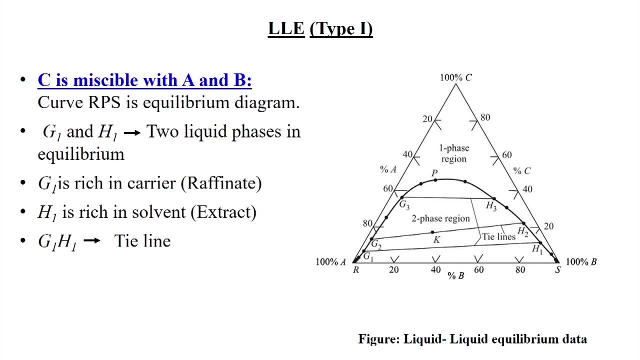 Now we will be discussing about this type 1 and type 2, where this we can say this one liquid-liquid equilibrium is: Say C is miscible with A and B in all proportions. we can say this one all proportions for any proportion. so we can say this one A and say C will be miscible in all proportions. 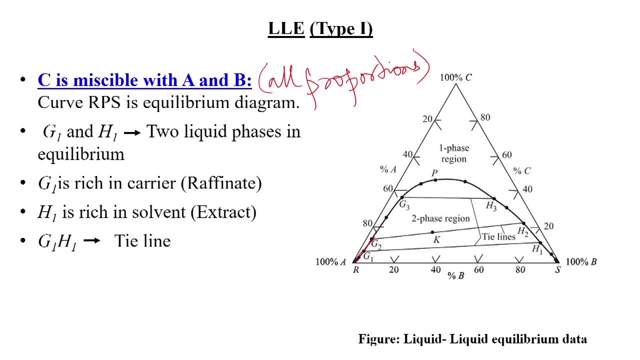 Like this. we can say this curve, this we can start from R to P to S. So in between this one, we can say this one, this is binary phase zone. So here you see, we will be discussing this, We will be discussing in detail about the binary phase. or we can say this: one, two phase. 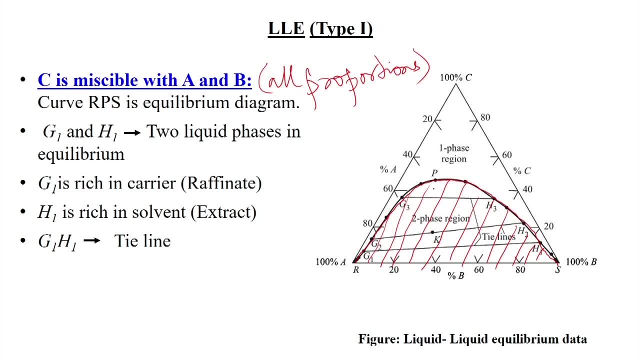 region where we can say this one from R to P. So that is actually we can say this: 100 percent. A means this is we can say this: one: carrier solvent, So carrier solvent, reach zone. so this is, we can say this one: a raffinate arm. 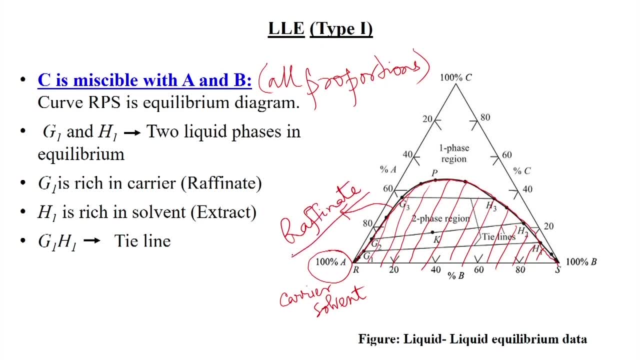 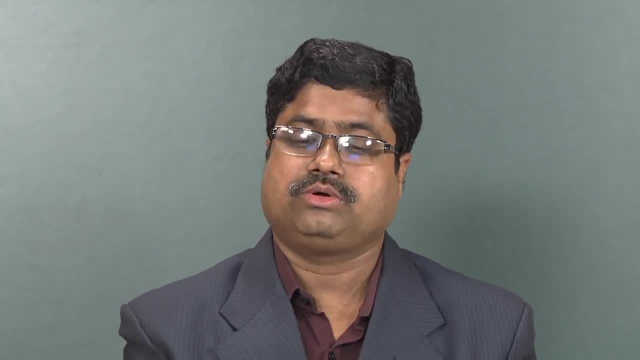 We learnt this one: that whenever the exhaust stream will be there, Where less amount of the solute will be present, so you see the solute also will be very less amount, because 100 percent is here, so definitely this less amount of the solute will be present. 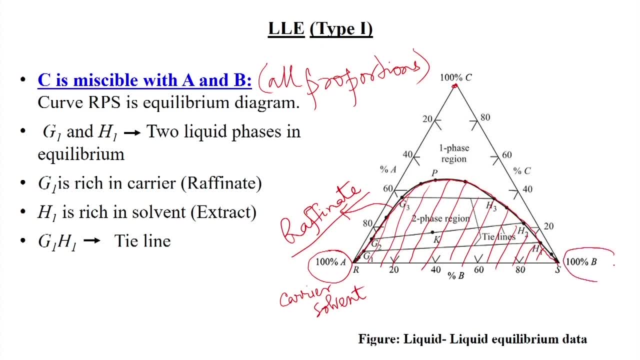 in the carrier, solvent. and this B is actually, we can say this one- extracting solvent. so B is extracting solvent. so here, from P to S, that we can say this one raffinate arm, that is say extract arm. so this one, we can say this one from R to P, this is raffinate arm. 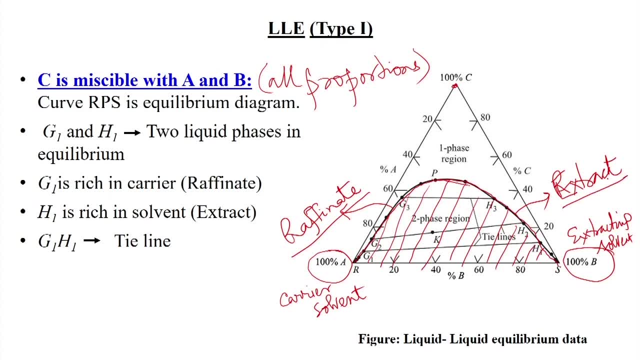 from P to S. this is extract arm. So this suppose for this two phase in this two phase equilibria line. so suppose from G1 and H1, suppose G1 and H1, this is connected with one tie line. so this: two liquid phases. 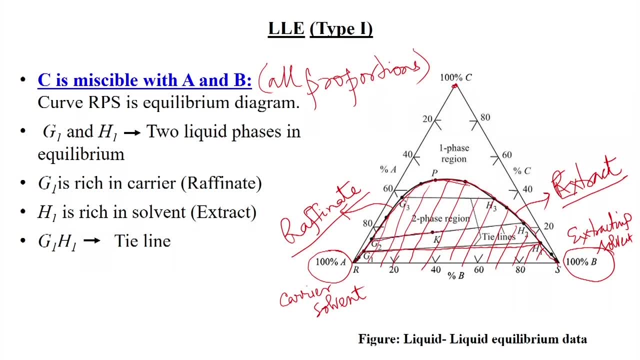 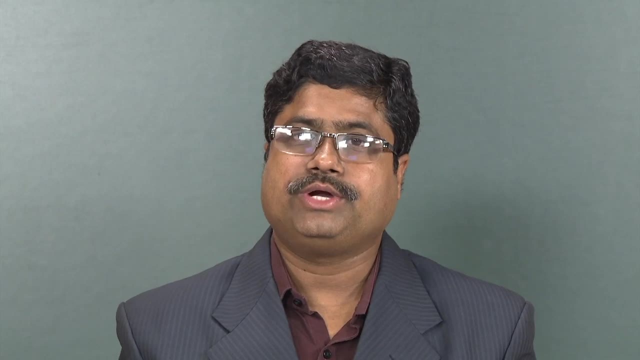 are in equilibria and from, suppose, from G2 to H1. That is also in the equilibrium. suppose we have added this one extracting solvent in the feed and we have mixed this properly. suppose this K is one particular point and we can say this one K is a particular, we can say composition if we wait for a while or we. 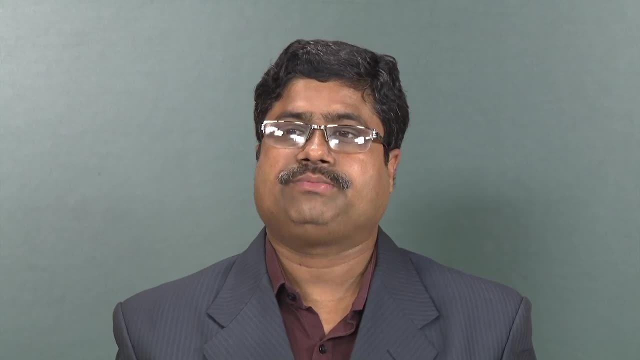 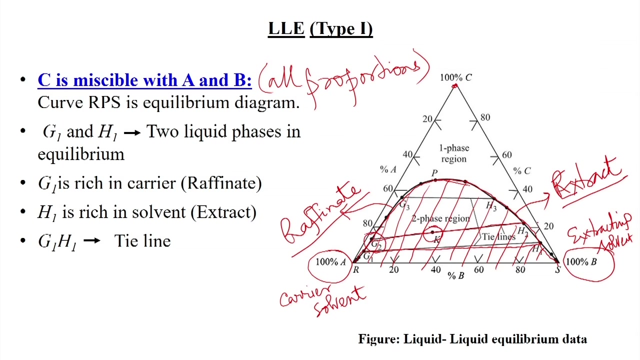 can say this one: if we allow this entire system to be separated from each other, then it will be separated like this with G1, G2. composition, it will be in the raffinate phase and H2 composition in the extract phase, and that is why G2 and H2, that is, we can say this one tie line. 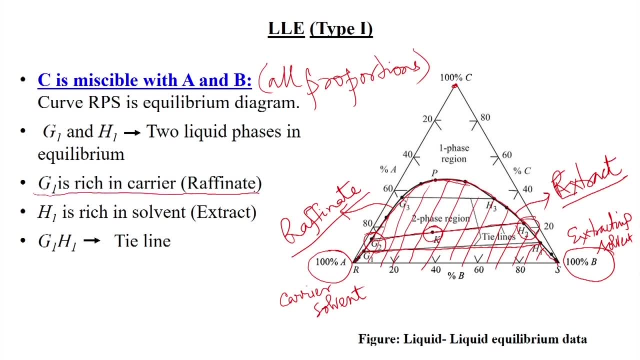 So G1 is rich in the carrier. we can say this one G1, G2, both are rich in the. we can say this one raffinate and H1 is rich in the extracting. we can say this one solvent, that is called H1, H2, H3. all these are, we can say this one extract, and say G1, H1, G2, H2, G3, H3. 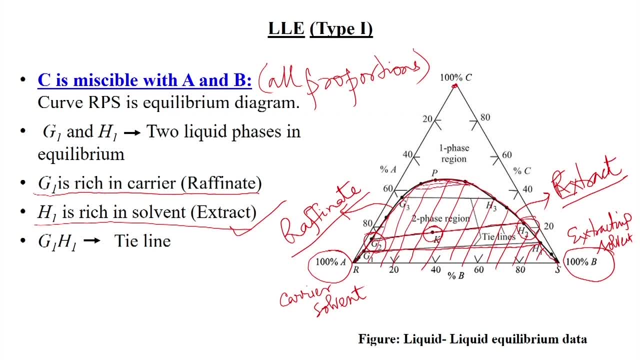 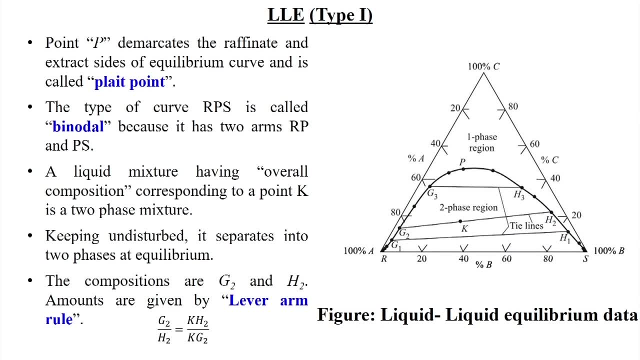 all these are. we can say this one: these are all tie lines. and then one point is there that is a common point, that is P. we say: this one is the plate point. we will be discussing in detail about that. And then this point P, that is, determines or demarcates the raffinate and the extract side. 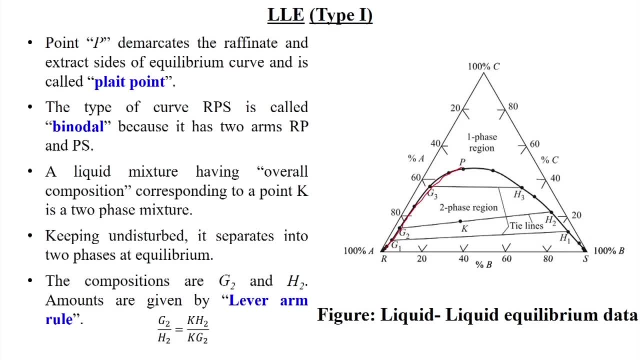 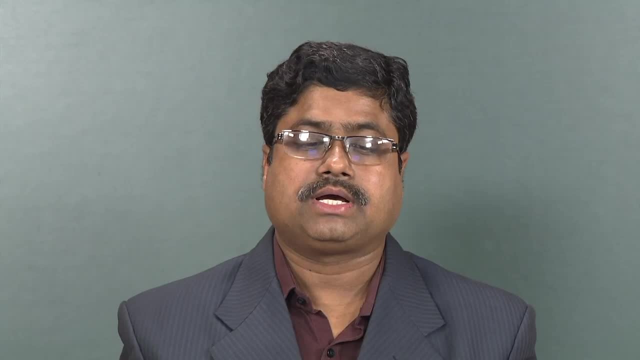 say I told that this one R P this part, you can see, We can say this one as this raffinate, raffinate arm and this is we can say this one extract arm. So these two, so this raffinate and extract sides actually of the equilibrium curve that 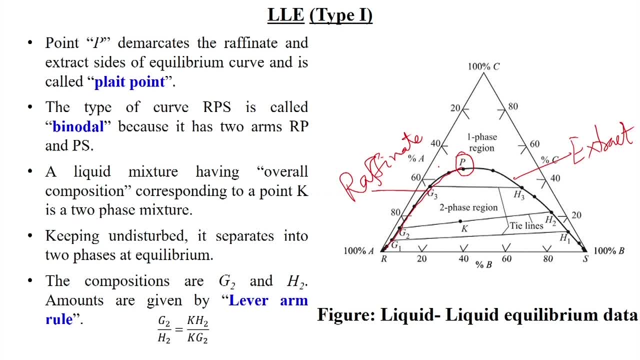 is called, say, P is called plate point, This type of curve, actually this R P S is called this binodal because it has two arms, like R P and P S, A liquid mixture having this overall composition composition. So this is the raffinate. 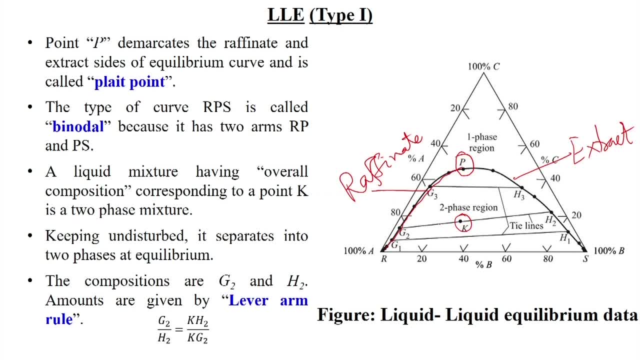 So this is corresponding to point K, suppose I told that. say this: overall composition. K is there and we are waiting for a long period of time so that these two will be separated into two different phases: liquid phases, One- we can say this one raffinate, and another, this one extract. 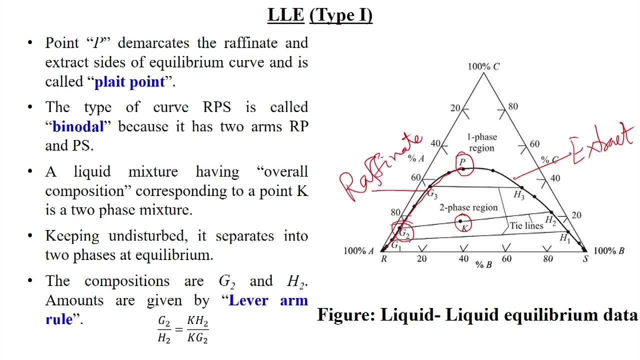 So this composition will be: G2 will be the raffinate phase, concentric composition, and H2 will be the extract phase composition. So keeping undisturbed it will separates into two phases. at equilibrium The compositions are, we can say this, G2 and H2, so this amount actually will be obtained by this lever rule, that is, we can. 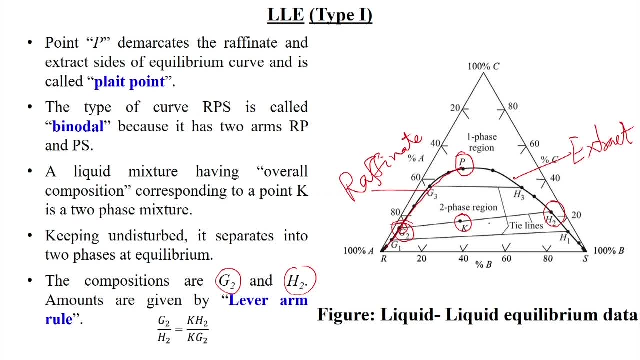 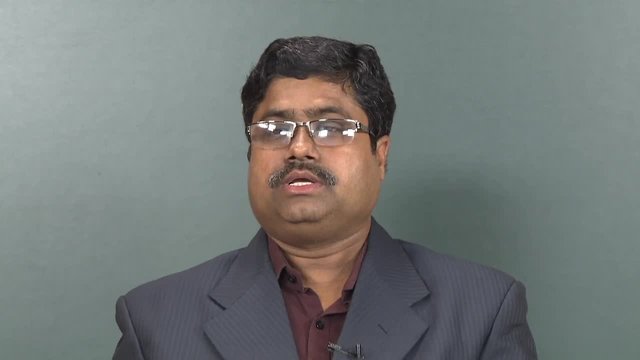 say this: one G2, G2 divided by H2, equal to say this one opposite arm, this KH2 by KG2, so this is, we can say this one: using this lever rule, we will be able to get the what will be the composition of the extract arm and the raffinate arm. or we can say this in: 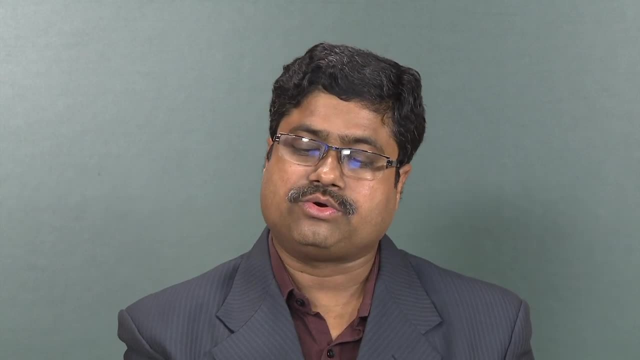 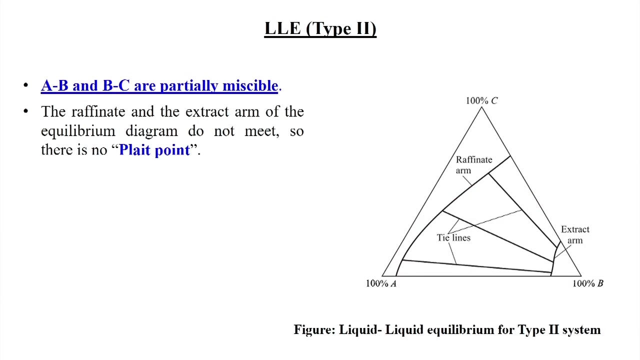 extract composition and raffinate composition, and it is actually controlled by this, what is called the tie line, The another type. what is? we told that this A, B and B, C are partially miscible. in that case, there is no flat point. so this raffinate arm will be like this and we can say this: 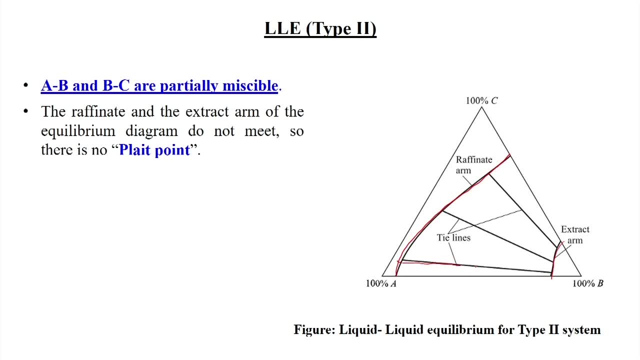 one extract arm will be like this, and then tie lines. all the tie lines are this one obtained in this way. so this is one tie line. we can say this one, In the we can say this B, C, the line where we can say 100 percent C is present, and also in between this A, B. 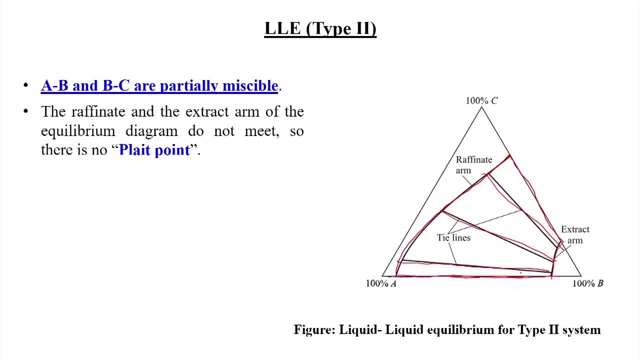 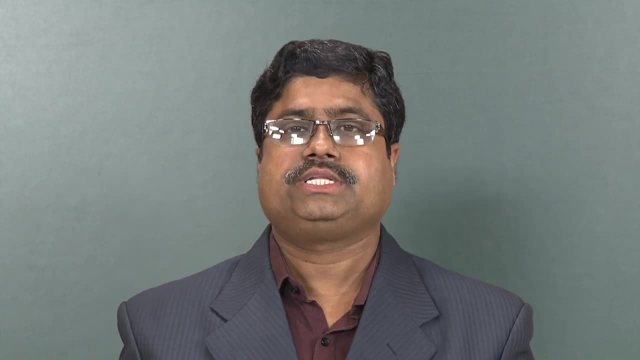 this line. this is also one tie line, so here there is no flat point. but you see we will be also discussing this one. if we do something modification here also, we will be able to get the tie line flat point in this, that type of type 2 system or we will be discussing. 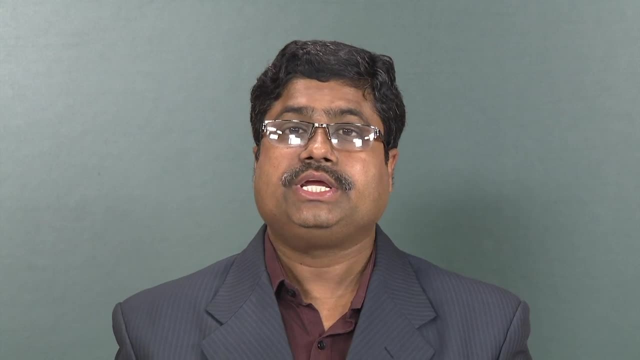 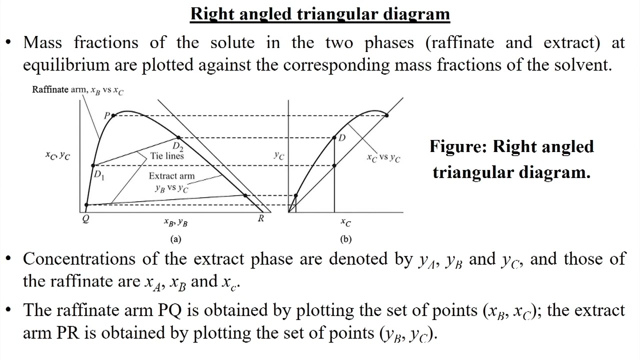 this one in detail about that: the conversion of type 2 system into type 1 system. So we will be discussing in detail also on that. Now we will be this one drawing this right angle triangular diagram from the, we can say this one ternary diagram. 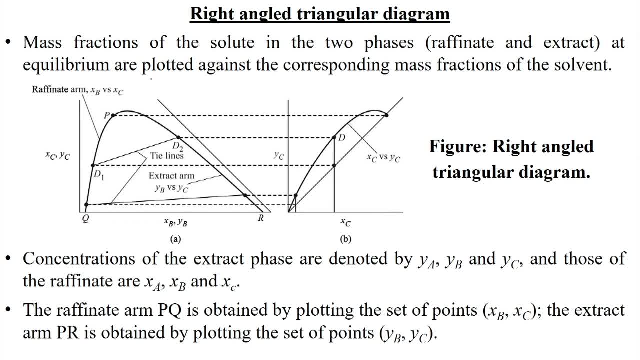 So let us take, say we have drawn this, we can say a small part of this ternary diagram. just we have not mentioned the C part, actually this where the C, 100 percent C, is present, that part, because you see, in the extraction process also we will see that this 100 percent. 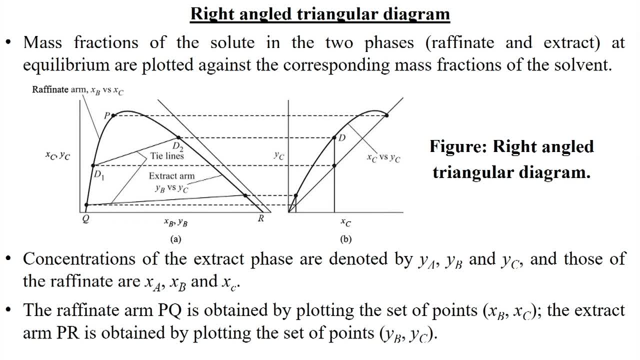 C cannot be this one separated, Separated using this one. so that part actually is not so important. so we will be discussing this part. where the equilibrium is means binary phase zone. is there? suppose here actually this binary phase is there? we told that this binary phases are like this, where the we can. 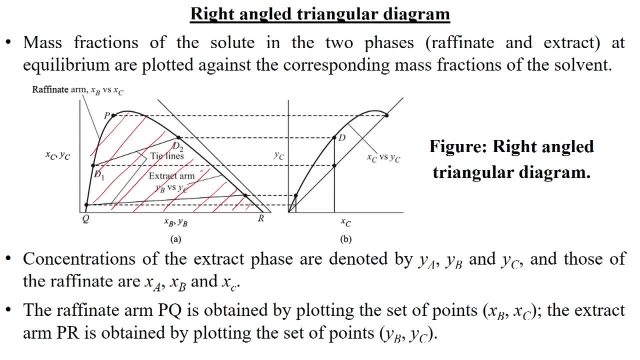 say this one: C is miscible in any proportions into both A and B, or we can say carrier solvent and the extracting solvent which has this plate point Like this, the mass fractions of the solute in two phases, like this in the raffinate and 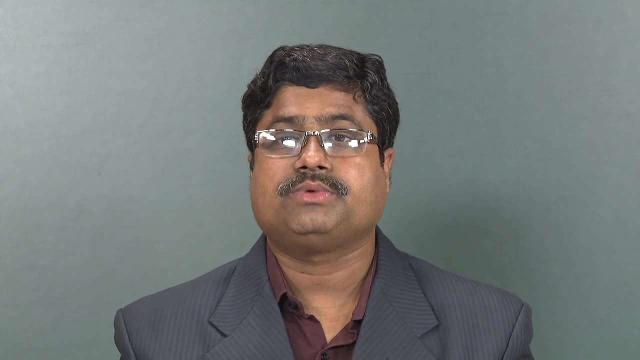 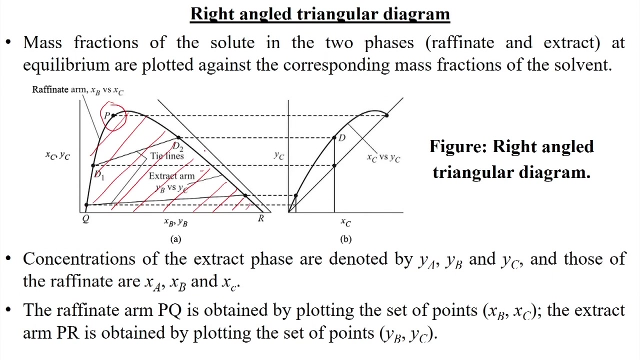 extract at equilibrium are plotted against the corresponding mass fraction of the solvent. So that is, we will be drawing also from this, we can say this one right angle triangular diagram. we will be able to get the say, we can say this one- equilibrium values of this Xc and Yc. how we will be drawing this one we are discussing in detail like this: 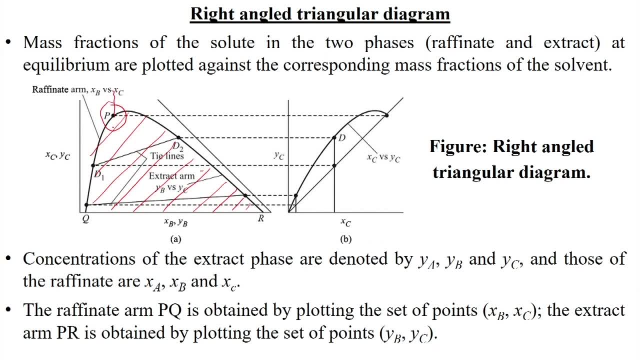 So concentration of the extract phase are like this: suppose this one up to this, we can say this one. so that will be say, from Q point to P point we can say this one will be XB versus XC. that is why that is XB versus XC. and after: 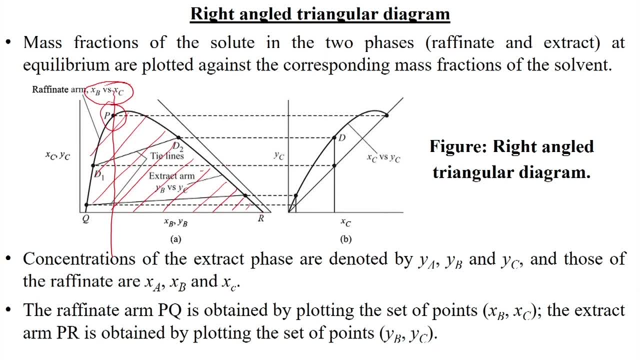 that point P to R. it is actually we can say this: one YB versus YC. that is, YB versus YC is there, But whenever we will be drawing one tie line. you see this. all these are actually drawn from the tie line data. suppose this P has this. we can say this: one P will be lying for. 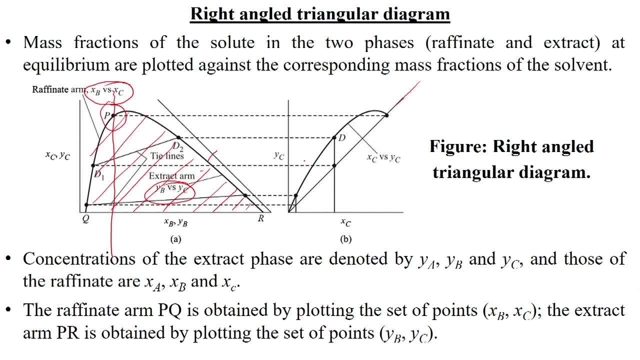 in the say diagonal of this XC and YC, because you see, the P is the common point where we can say this one here, you see, the in plate point XC is equal to YC. that is why we say this one is the tie line, the plate point. 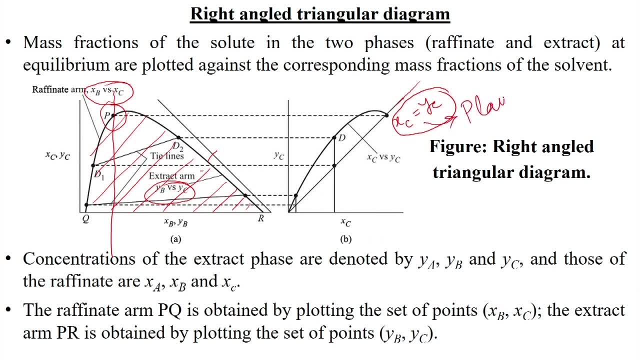 So this is corresponding to plate point, this plate point, and whenever we will be drawing any point, So any tie line, suppose this is the one tie line. so from here what will be doing? this is corresponding to, we can say this one, this XC and YC. also, suppose this is YC and this. 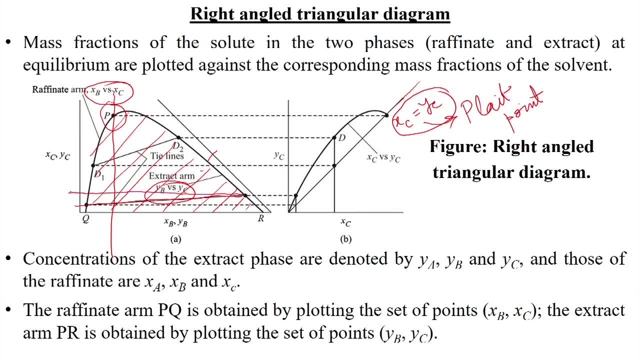 is XC. so that is why, whenever we will be coming to this point, that is, we can say: this one, this is YC, this one is YC and corresponding value: this one is called this Corresponding value. actually is called this XC, this is XC. 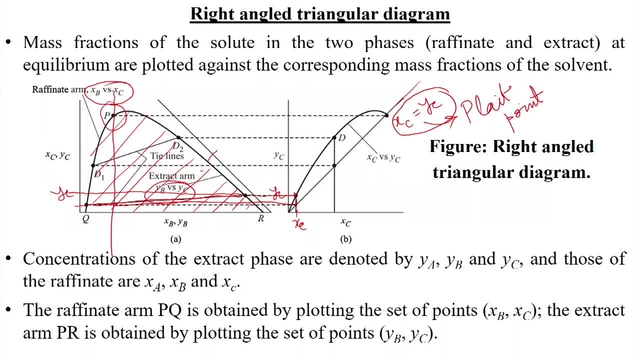 So whenever the equivalent to XC, whatever the YC value, is there, from this tie line we will be able to get this one: say: we have this XC and we have this YC. this is one cutting point. Let us take this tie line here also. you see, this one is XC value will be coming to this: 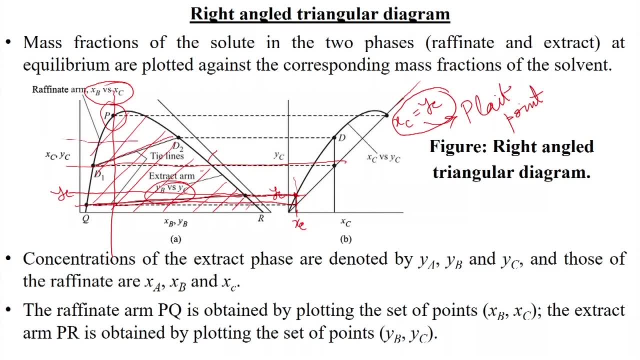 diagonal line and corresponding. this actually is YC value, Means say how we will be getting this one. we will be extending this XC and up to YC value then whenever it will be meeting one point, so that way for all the tie line values we will be getting this common points for any XC value. suppose this another YC value is. 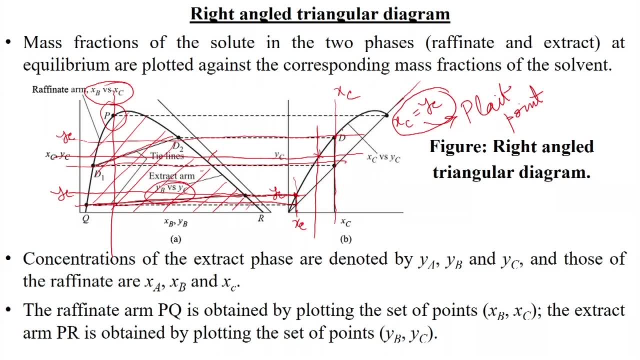 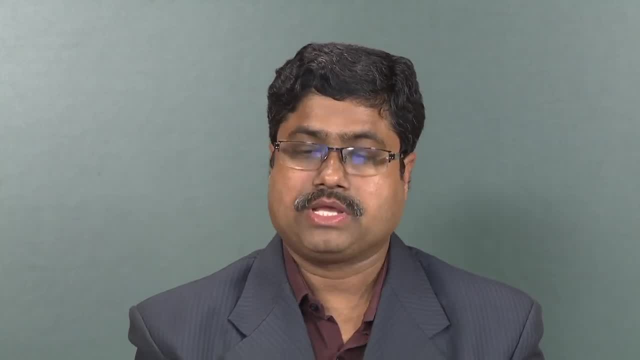 there. So using this one, we will be getting the common points like this way. so then we will be able to get the say we can say this one equilibrium line, And whenever we will be joining this equilibrium line, we will be getting that, the corresponding to XC value. what will be the YC value? 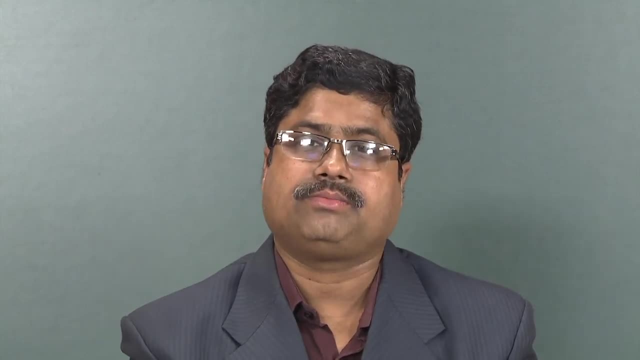 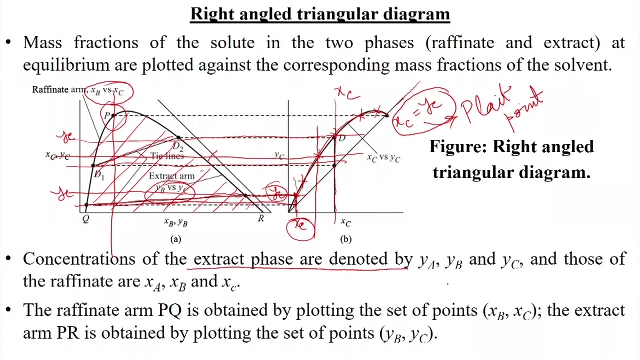 And we will be frequently. we will be drawing this equilibrium curve for the extraction calculation and say we can say this one for the extract phase. in all the cases we will be denoting YA, YB and YC and those are the raffinate phase. we will be taking this one. 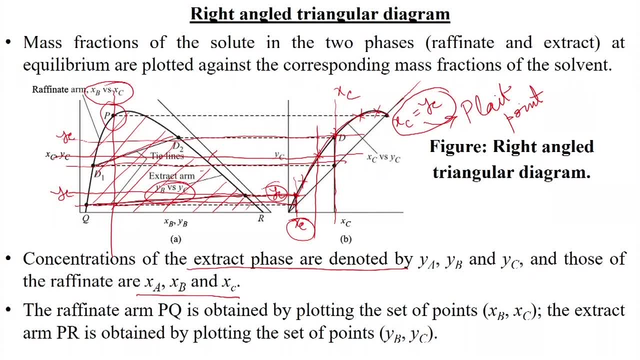 the XA, XB and XC. So these are the common notation values. So this is the common notation values. So these are the common calculations actually we will be using for the entire extraction calculation. Then the raffinate arm PQ is obtained by plotting the points like this: XB and XC, suppose this. 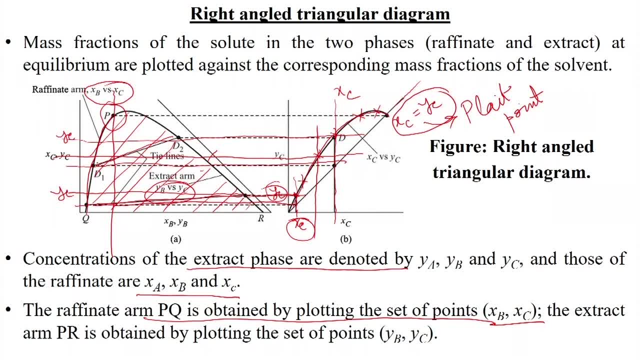 raffinate arm will be getting this one by plotting this XB and XC and extract arm will be getting from this plate point by plotting this YB versus YC. so we will be getting this one. So raffinate arm will be getting by plotting this set of YB versus YC. 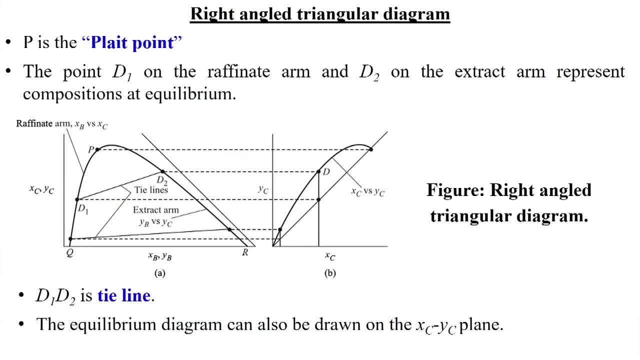 So the here also this P is the plate point and point D1 actually on the raffinate arm and D2 on the extract arm represent the composition at the equilibrium that we told that say whenever we have this D1 and D2, say from D1 we can say this one, nothing, but this is the XC value. 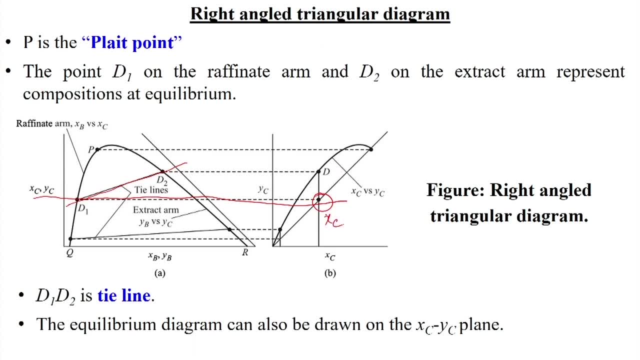 so this is- we can say this- one corresponding to XC, and so whenever this we have, this XC, we will extend this one. and from here you see, this one YC will be getting- suppose this is YC value- whenever it will be cutting, so it will touch this line. 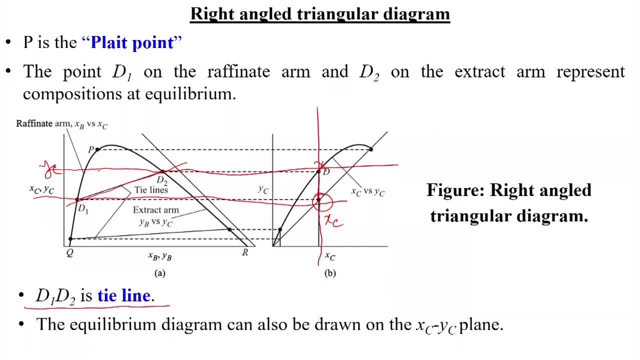 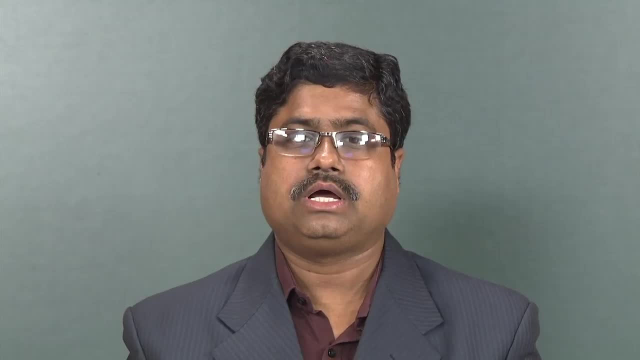 So D1, D2, that is the tie line. So all the tie line values, actually all the tie line data points are there and from there we will able to get the. we can say this: one equilibrium line Also, equilibrium diagram can also be drawn on the XC, YC plane also. that also we can. 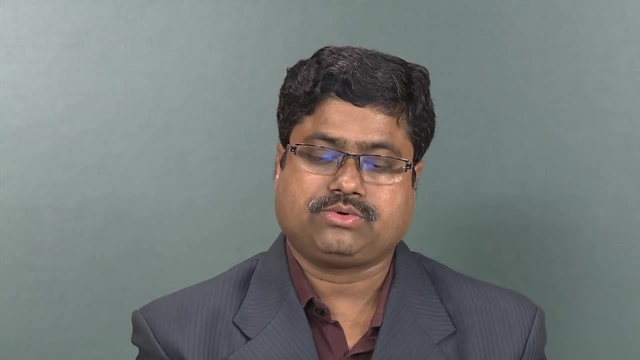 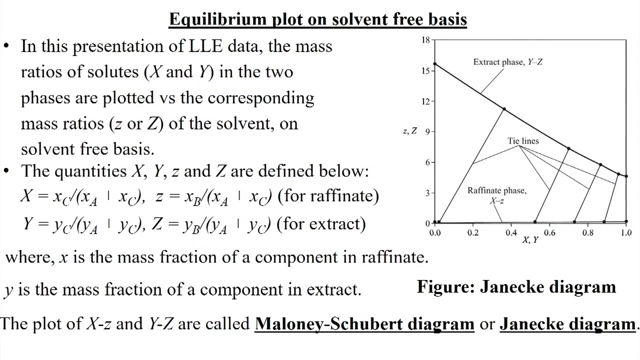 say this one will be discussing this one, so means this one or this one, anything will be okay for the table. Yes, this one, what is called general calculation, And in another way also. that is also very convenient method of this equilibrium plot on the solvent free basis, like this in this: 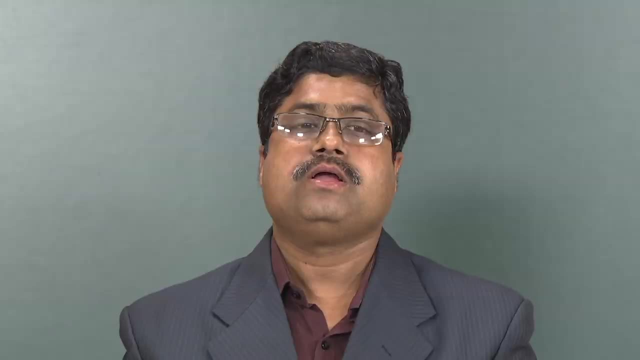 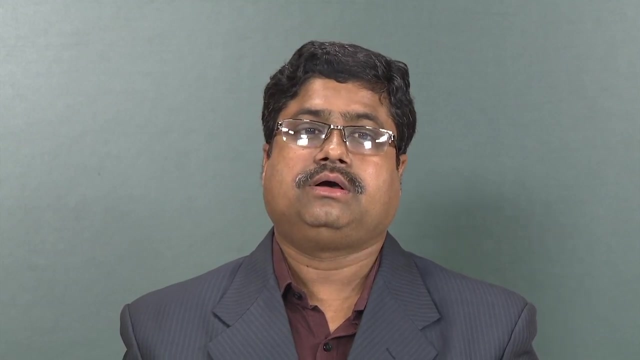 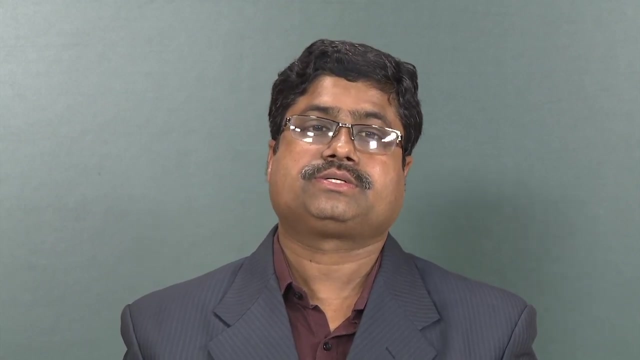 presentation of this liquid-liquid equilibrium data, the mass ratio of the solute- we can say this one in: x and y in two phases, like this, we can say this one: are plotted like this: we can say this one for capital X. we can say this one: capital L, x and small z will be in. 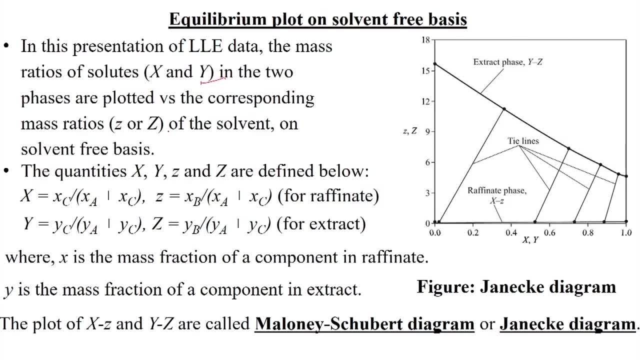 the raffinate phase and capital Y and capital Z in the extract phase will be used. this one, so that is, we can say this one. all the values are in the solvent free basis. we will be discussing the advantages of the solvent free basis calculation also. 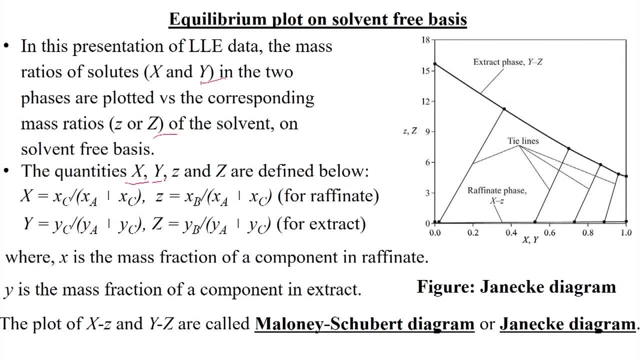 So the quantities capital A, X, capital Y, small z and capital Z are defined like this. So we need to remember this one: capital Ax is equal to small xc by small xa plus small xa, and where this small z is equal to small xb by small xa plus small xc, whereas this y that 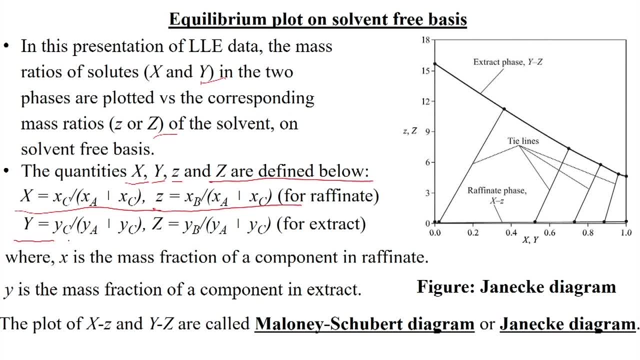 is in the. we can say this one extract composition that is equal to yc by ya plus yc, where capital z. that is, we can say this one: yb by ya plus yc, capital X and small z. that. we can say this: one that is in the raffinate phase composition. 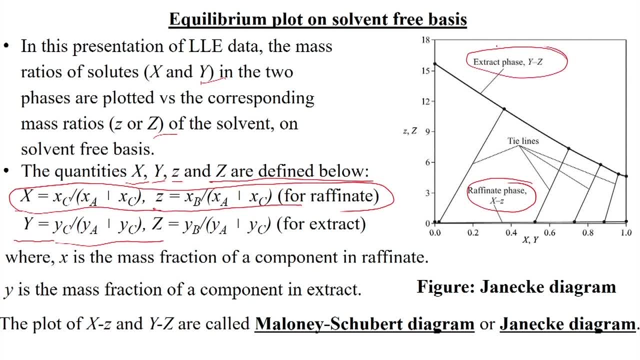 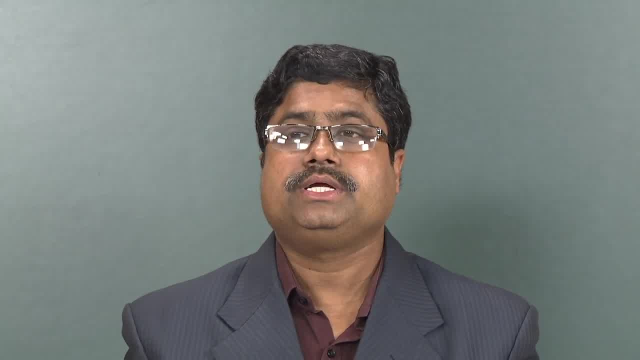 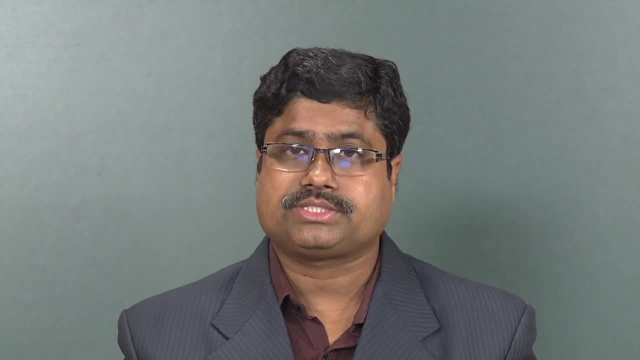 and in extract phase, that is capital Y, capital Z. So we will be calculating this one, we will be solving one small problem to understand that whenever we will be drawing this equilibrium plot on the solvent free basis and from there actually we can see all the calculations are very simple. 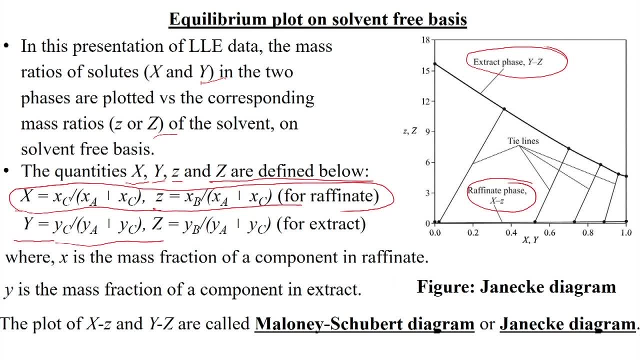 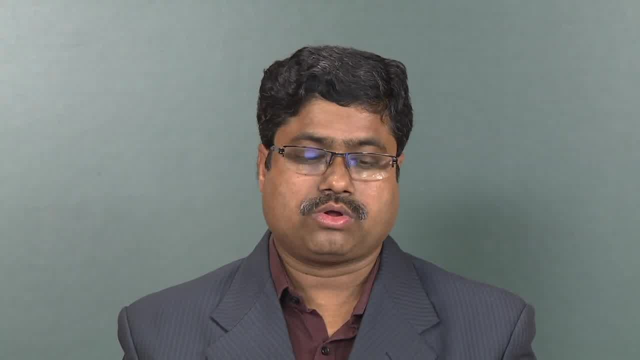 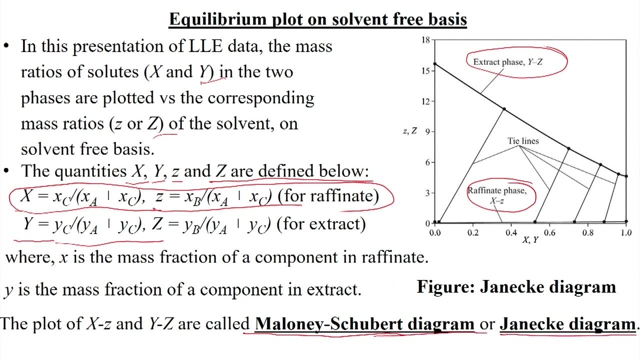 This diagram, that is, we can say this: in the equilibrium plot of the, we can say this extract arm and in the raffinate arm is called this Janicki plot. or we can say this: one Meloni-Savart diagram also. or we can say this: one Janicki diagram. 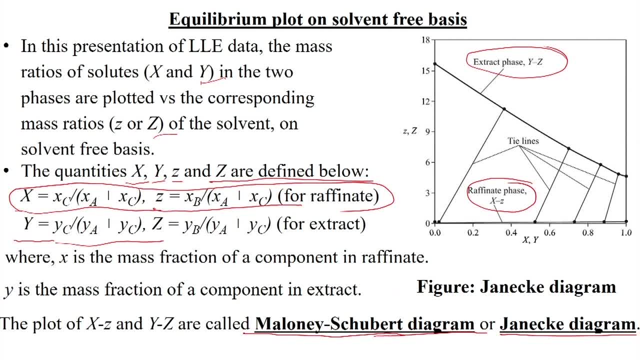 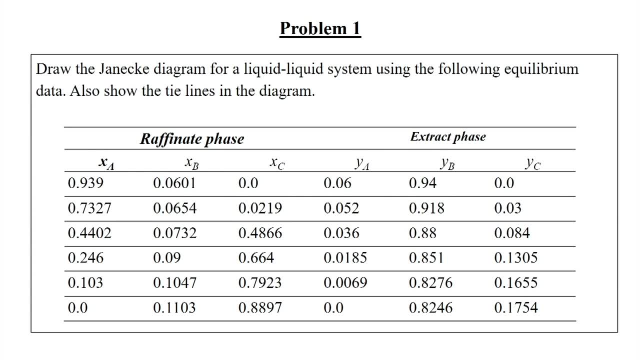 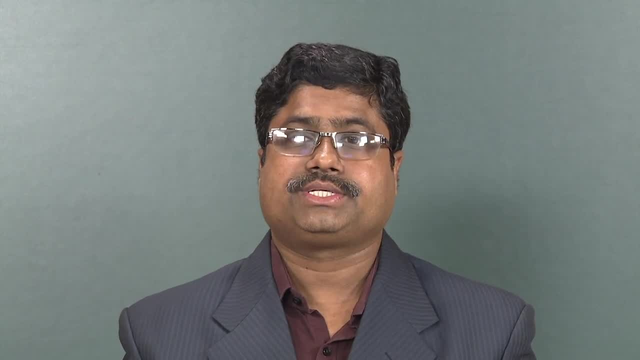 So it is very convenient way of this one calculation for the extraction process. Like we say, we will be solving one problem, very simple problem actually, how to plot this one, and from there we will be able to know that, how, this, we can say this: one equilibrium. 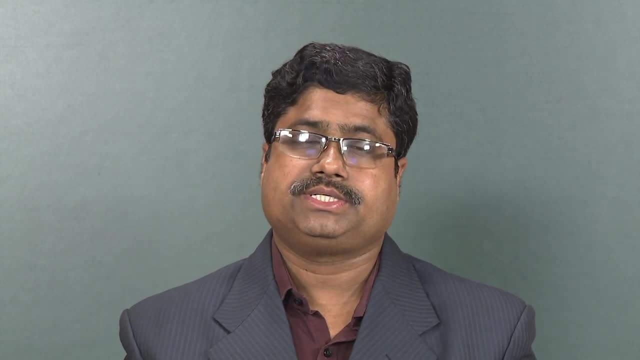 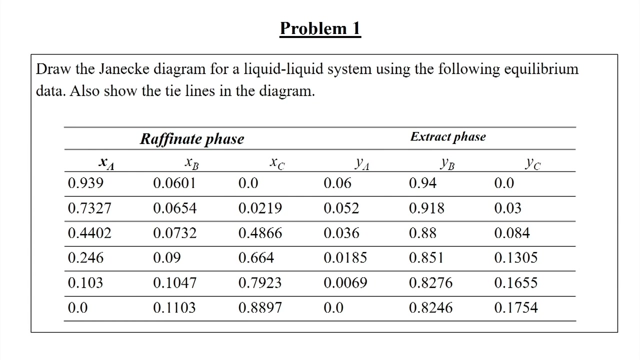 plot is done on the solvent free basis. The problem is that draw the Janicki diagram for a liquid-liquid system using the following equilibrium data: Also show the tie line in the diagram Like this in the raffinate phase say we have this: XA is equal, to suppose, 0.939. where is 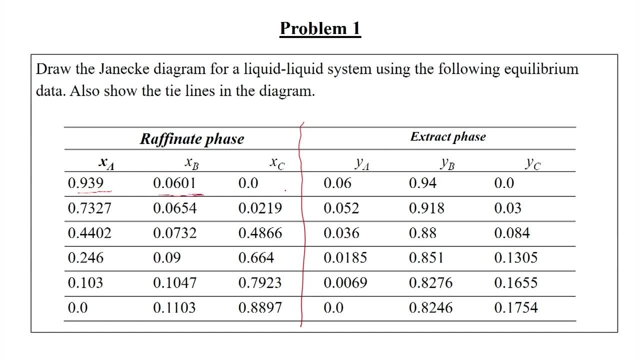 XB is equal to 0.0601 where XC is equal to 0. so in one point, that is, we can say in the left hand corner, where we can say this, only the extracting solvent. and we can say carrier solvent is there, there is no solute like this, and say this one XA is going on decreasing. 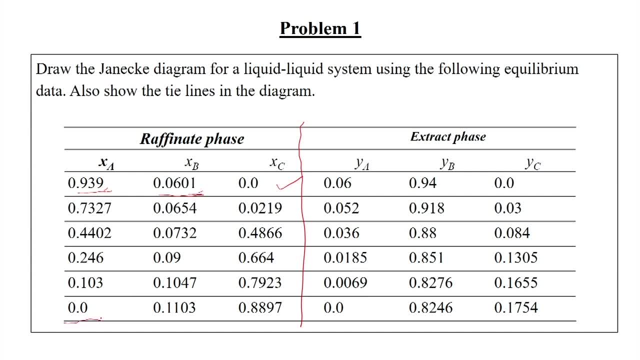 slowly and somewhere we can say this one no extracting solvent is present where this XB is there and XC value means we can say the solute contribution is maximum in this case. So this is the solution. So in the raffinate arm where 0.8897 comparison is there. 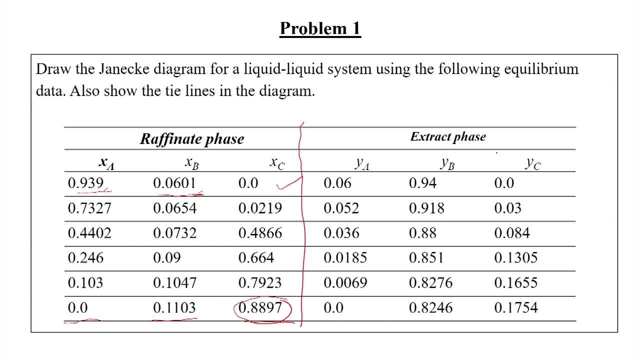 So if we add all this we will be getting 1 and for extract phase, say we have this one. we can say whenever this 0.06 YA is there, and say we can say this YB is maximum 0.94 so and say like this is the right hand corner actually, and we can say this: one YC actually. 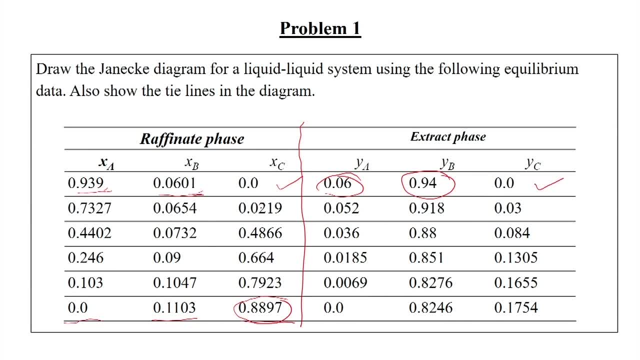 there also is 0.. So whenever we will be plotting This one in the raffinate arm and extract arm, we will be getting one common point like this: we will be getting this plate point also. so we will be coming to that point, this plate. 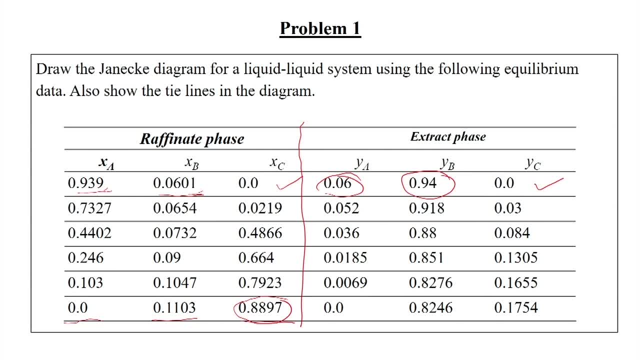 point also we will be getting, but we will be doing this. one in the Zernike diagram means we will be plotting this one in the solvent free basis. So for that we need to calculate this. four parameters like this: capital, X, small, z, capital. 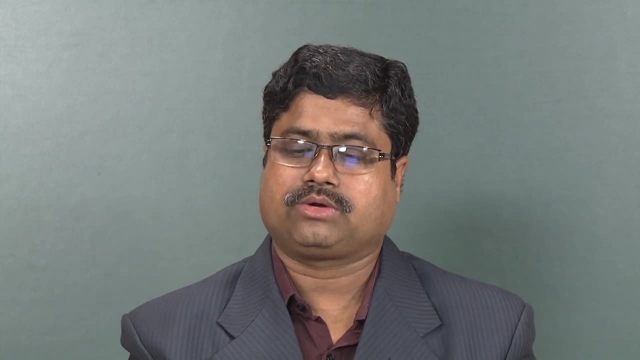 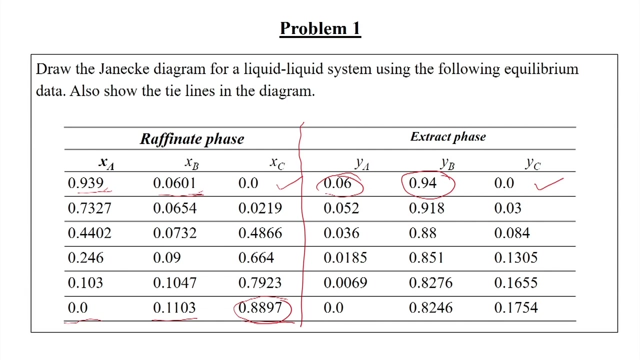 Y, capital Z. So this four will be there. So this four will be there. So this four we will be calculating. then we will be plotting this raffinate arm and extract arm in the say we can say this one solvent free basis in the equilibrium plot. 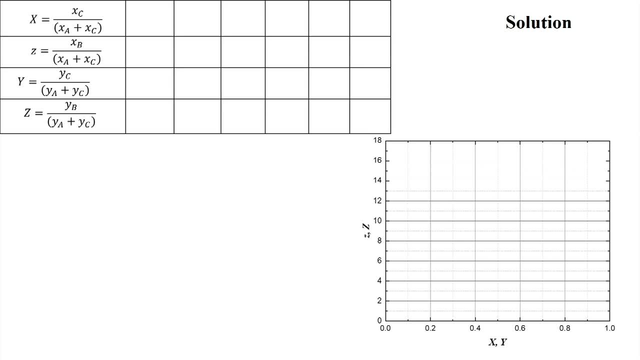 So now we will be calculating this one for this, all this data points. we will be calculating those like this, what we will be doing for this. suppose for first data point, like this: for the raffinate arm we have, X is equal to 0.939, XB is equal to 0.0601 and XE is equal. 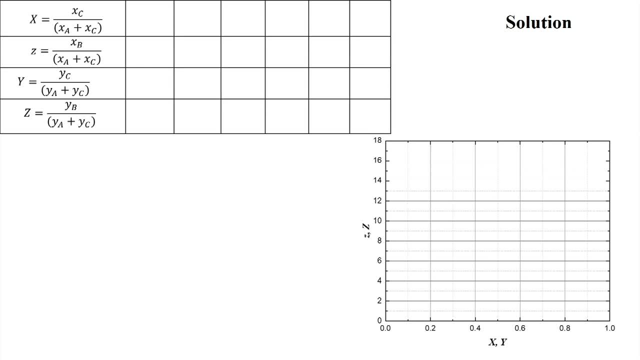 to 0.939.. So this is the raffinate arm. So this is the raffinate arm. So this X is equal to 0.6 by XC is equal to 0.. So we can say this one: as this X value is equal to XE, by XA plus XE, so will be 0 by 0.939. 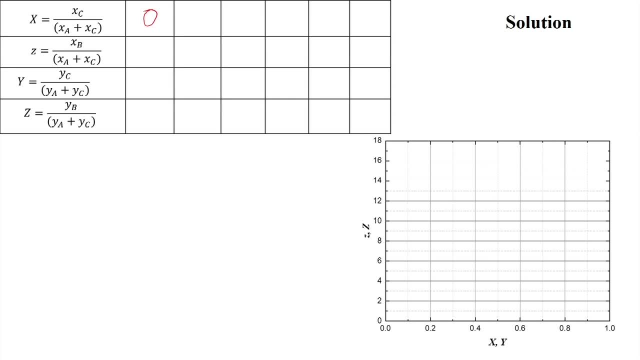 so it will be 0 like this For second, this data, point 0.73, this one, what is called for XE, is equal to 0.0, 219 divided by 0.7327 plus 0.0219.. So it will be coming as we can say, 0.219.. 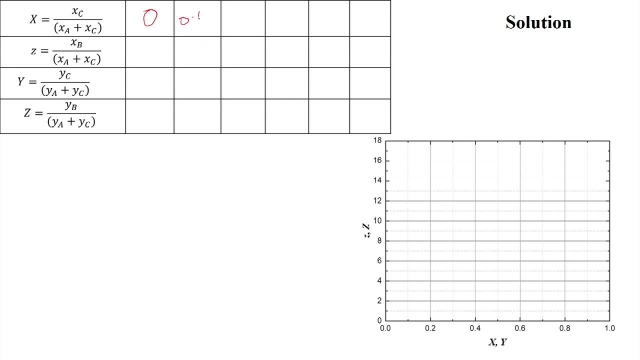 So this will be 0.219.. So this will be coming as 0.219.. For the third one, like this: 0.4866 divided by 0.4404 plus 0.4866, it will be like this: 0.525. and for the next point, like this: 0.664,. so it will be like this: 0.73. and for 0.7923, 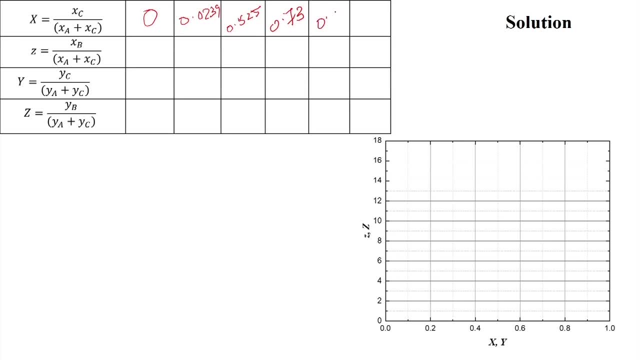 we will be getting this one 0.885.. And for 0.8897 we will be getting 0.192.. So it is like this: Then we will be getting this one as 0.8897 by 0.8897, that is, we can say this one we will. 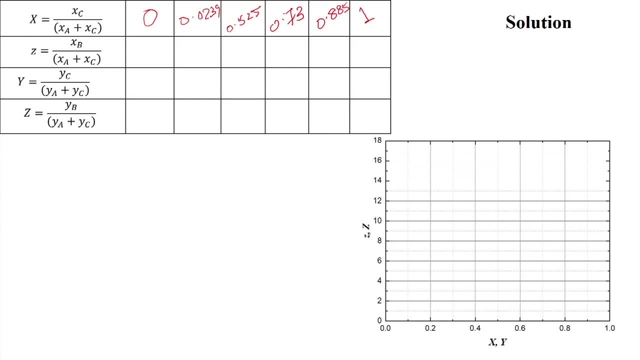 be getting x equal to 1.. For Z calculation also, we will be following the same xB divided by xA plus xC. suppose for first point, 0.0601 divided by 0.7327 plus 0.0219, so we will be getting as like 0.064. 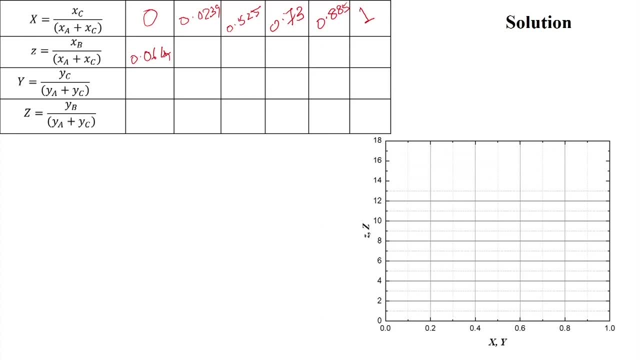 for other point, actually for the next point, we will be getting 0.067. for next point, actually we will be getting 0.079. this next point will be 0.099, then it will be 0.117 and then 0.124.. 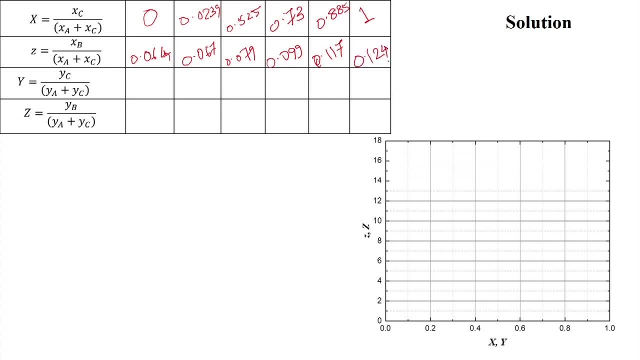 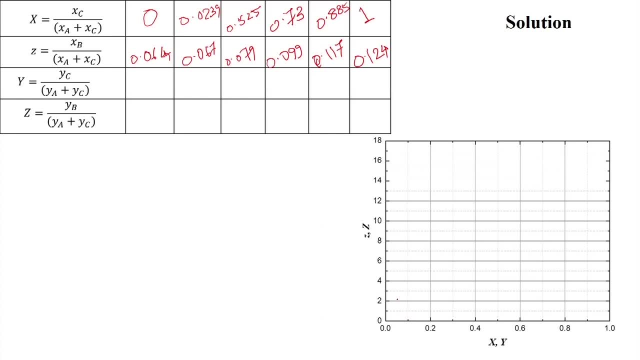 for raffinate arm. So we will be drawing this one in xy versus zz. plot actually this: all the values are. we can say this one whenever x will vary from 0 to 1. you see small z values are all within. we can say this one: 0.124. we can say that is almost. we can say this one will be in the 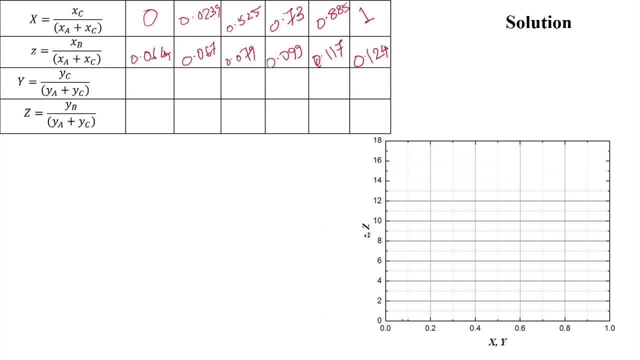 line of this ZZ. this one axis means you can say it will almost along the XY line And for extract arm actually say we can say these two: this one points will be for raffinate arm. Now extract arm actually will be calculating like: Y is equal to YC by YA plus YC, like this: 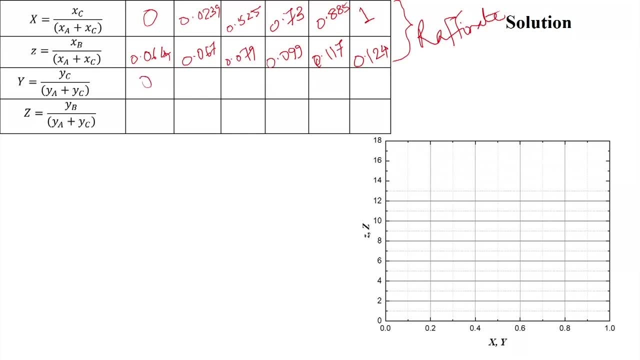 YC is equal to 0, so definitely this first point will be 0. then we have this for second point. we have this: YC value is 0.03 divided by 0.052 plus 0.03. that is we can say we will. 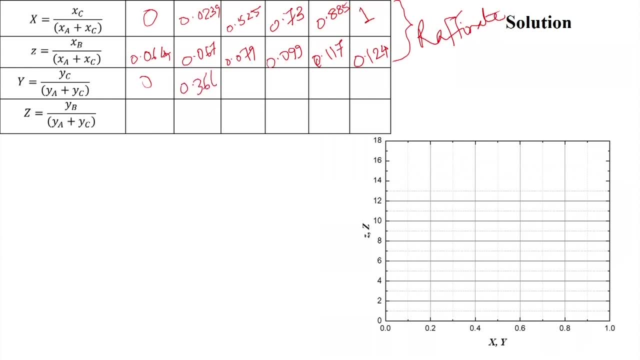 be getting this 0.366.. And the third point will be like this: for third point, we have this 0.084 divided by 0.036 plus 0.084, so that will be coming as 0.736.. And the next point will be 0.876, and then next point will be 0.96. and the last point. 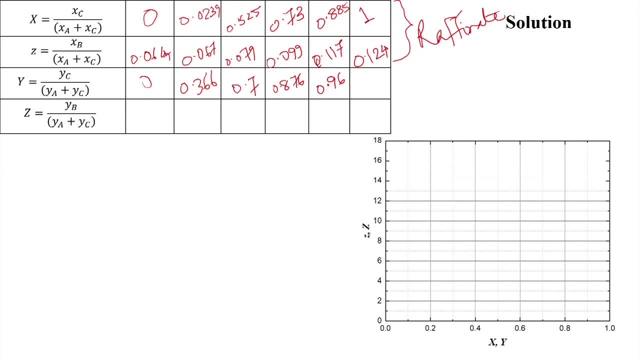 will be point this one: YC is equal to 0.1754 divided by 0.1754, as YA is equal to 0. so then it will be like this: 1. Corresponding to capital Z value, that is, we will be starting with this. 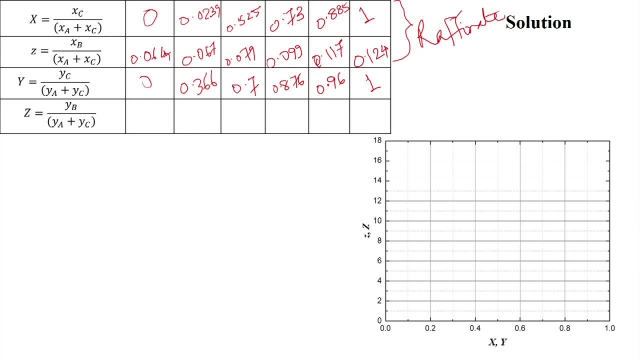 minimum, So the middle values of like this YB. so it will be work like 0.94 divided by 0.06. so 0.94 divided by 0.06 it is coming as 15.67.. Then second value will be 0.918 divided by 0.052. 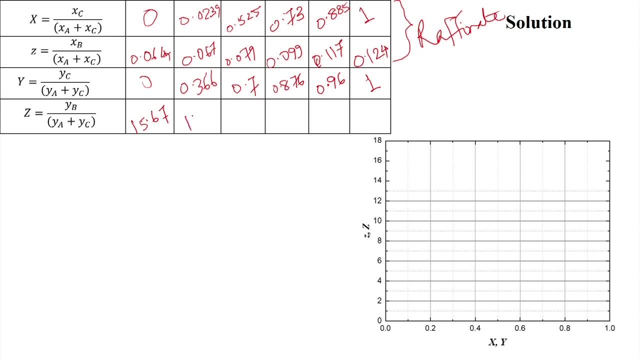 plus 0.03, that is coming out as 11.2.. For the third value: 0.88 divided by 0.036 plus 0.084, so it is coming out as 7.33.. The next value will be like this: in the same way will. 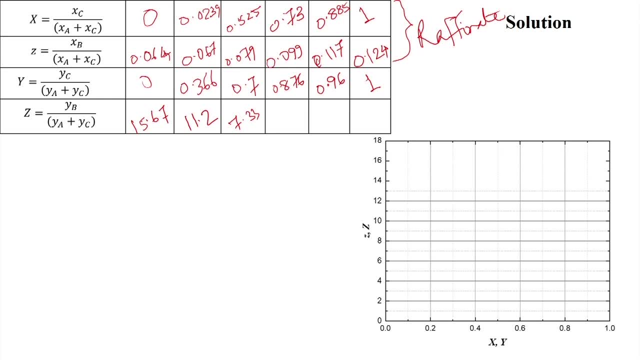 be calculating 0.851 divided by 0.0185 plus 0.1305. so it is calculated as 5.71,. then the fifth value is calculated as 0.8276 divided by 0.0069 plus 0.06 and5.. So it will be coming. 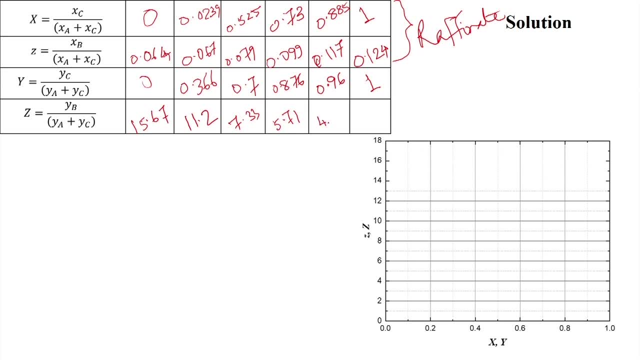 0.1655, that is calculated as 4.8. and for 0.8246 divided by 0.1754, it is coming out as 4.7.. So now these two points are for extract arm. so now we will be plotting these all this. 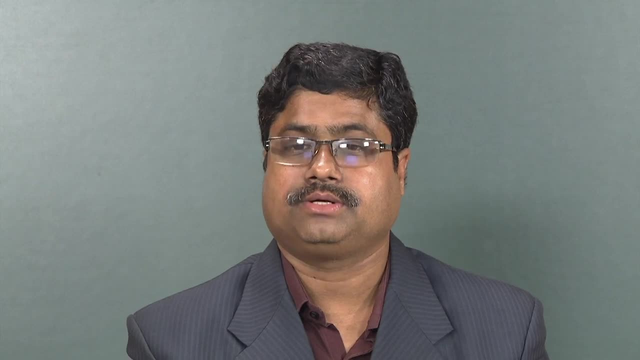 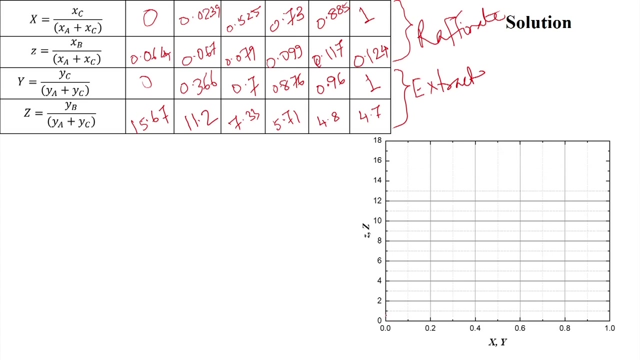 in the we can say this one xy versus zz plot. so for first we can say this one: whenever we have this x is equal to 0,, so this z is equal to small. z will be like here. so this is first point, then 0.0239, so it will be like here also somewhere here: 0.067, here also. 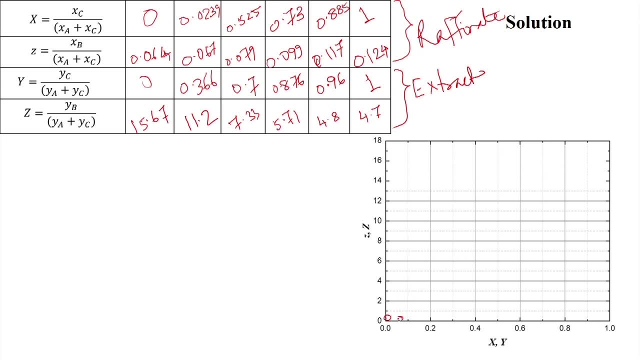 somewhere. it will be like this: Then say: then we have 0.525, so here actually it will be like this: for that: 0.079, so 0.525 means somewhere here. so it will be like this: 0.079,, 0.73 somewhere. here it is for 0.099,. 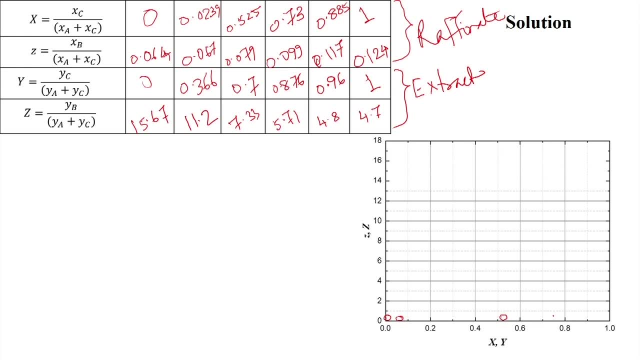 so it will be like this: so just below 1, like this 0.1, actually say here somewhere, and then this: 0.884. 0.884. 0.884. 0.885, like this somewhere. 0.885, here it is for 0.117, somewhere here, and for 1 it is. 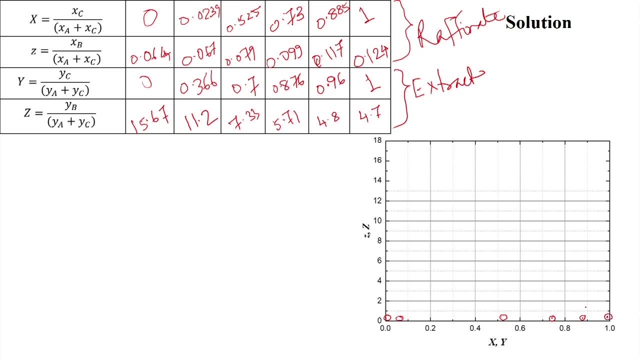 0.124. like this, so somewhere here. so if we plot this one, it is like touching this. we can say this xy axis like this, so this is, we can say this one, this raffinate arm, so this is raffinate arm. 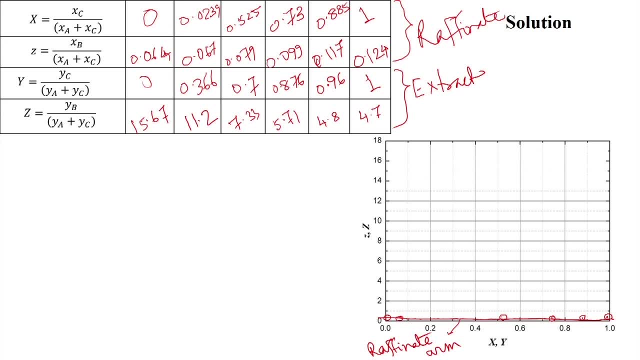 For extra term we can say this one will be getting, for y is equal to 0, so this one is y is equal to 0, so it is around 15.67, like this somewhere here, for y is equal to 0.366,. 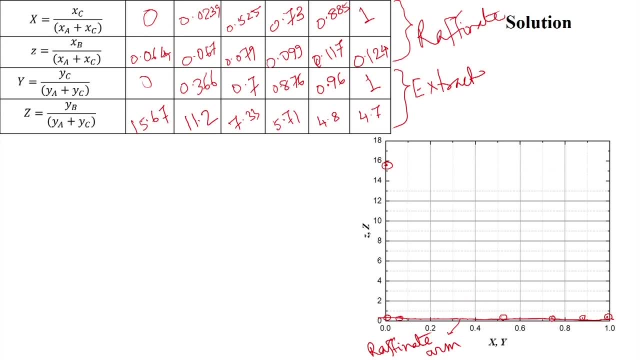 so somewhere here. so we will have this one for 0.366, like this: it is 11.2,. so it is like this somewhere here. So it is 11.2 like this. so this we have. so for this second one, for 0.7, it is 7.33,. 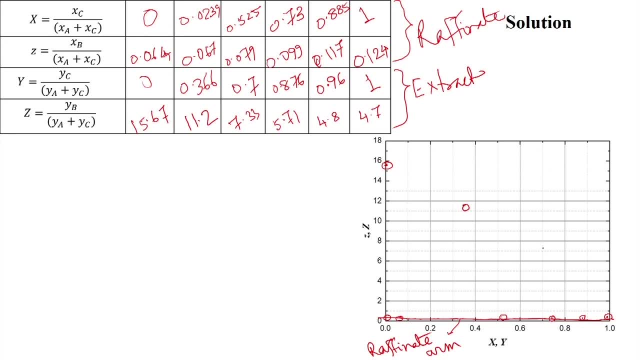 so it will be like this for 0.7, that is 7.33, 6, 7.33. like here for 0.876, like this for 0.876. it will be like this: 5.71.. So it is 7.33.. 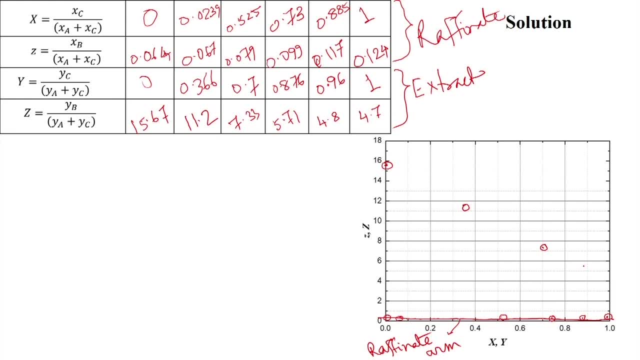 So it is 7.33.. So it is 7.33.. So it is around 6 here. so it will be like this: and for 0.96, so it is 4.8,. 4.96 means. 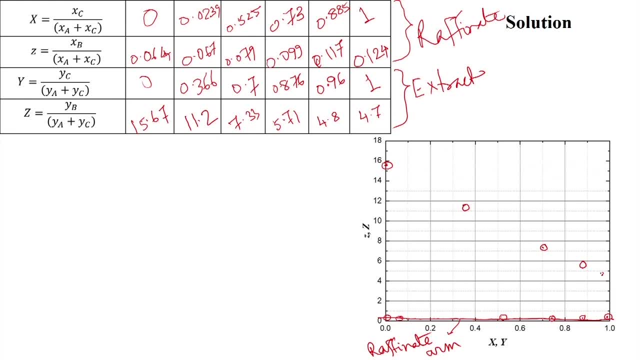 here it is 4.8, around 5 here and for 1 it is 4.7, so it will be like this: it is here somewhere. Now you see this one, we have this, all this line. if we draw, add all this or join all these. 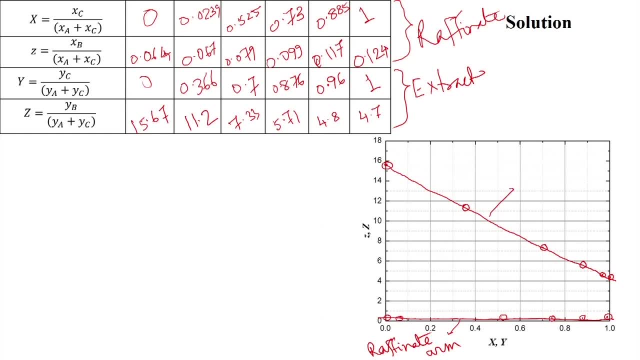 this or join all this, so we will be getting this one as the extract arm. Now we need to draw this. we can say tie line, so this one tie line. that is, we can say this one, this first point actually, so this is one tie line. we can say this one, so this: 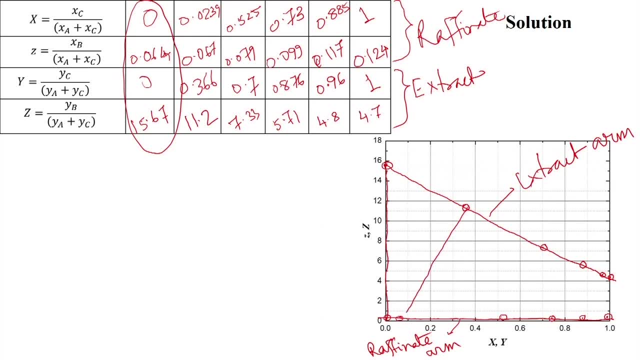 one, the second one, actually, you see, this is second tie line, then we have this third tie line, then fourth tie line, then fifth tie line, this is the sixth tie line. so all these are. we can say this one, all these are tie lines. so we can say this one, say raffinate. 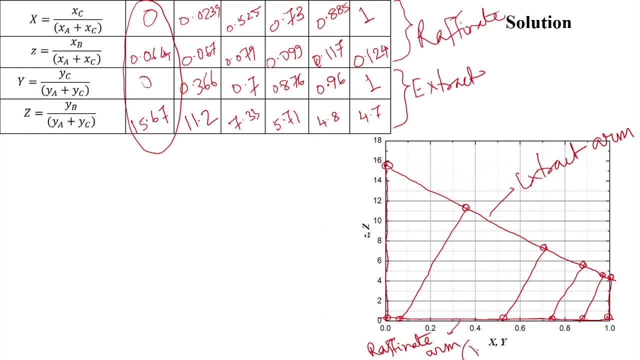 arm is nothing. but we can say capital X versus small z and extract arm is equal to capital Y versus capital Z, and these are all we can say, this one tie lines. so this is tie line. we can say this one: This is tie line. this is also one tie line. we can say this one: this is another tie line. 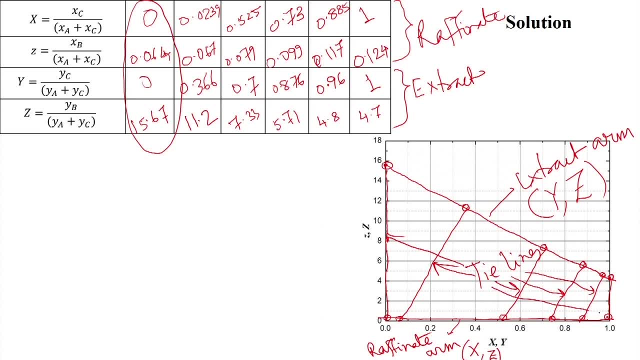 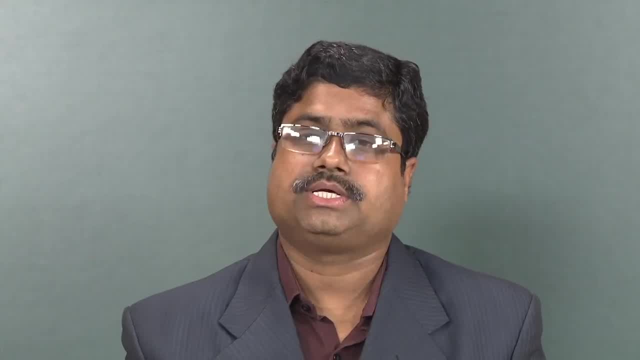 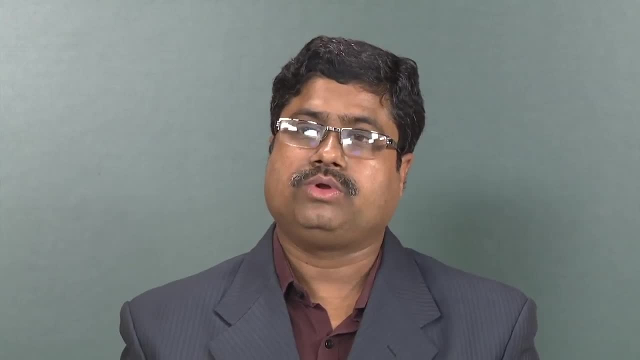 so this is one tie line, this is one and this is also one tie line. So now we have this one, the extract arm and raffinate arm. now actually we can say, using this solvent free basis equilibrium diagram, we will be able to calculate the entire extraction. 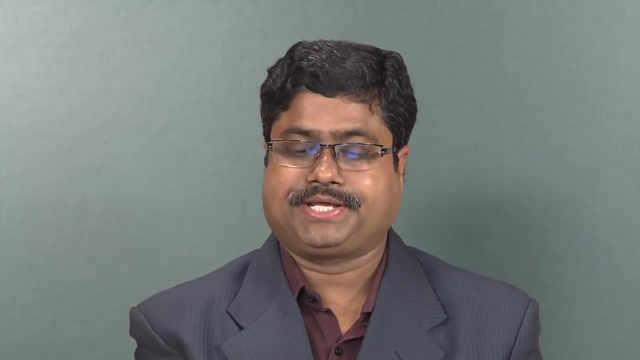 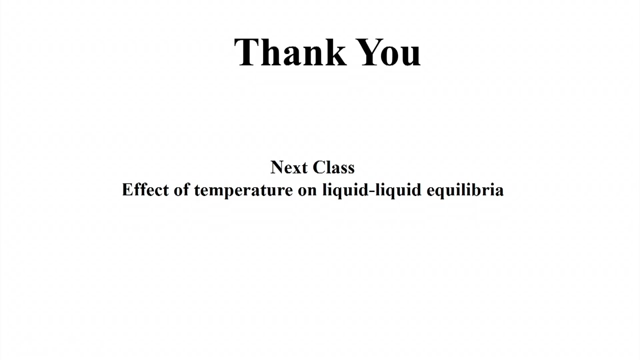 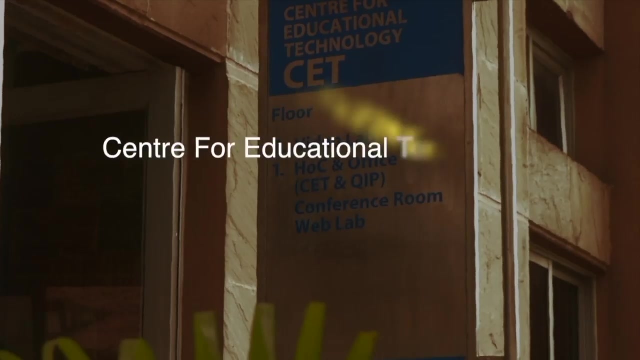 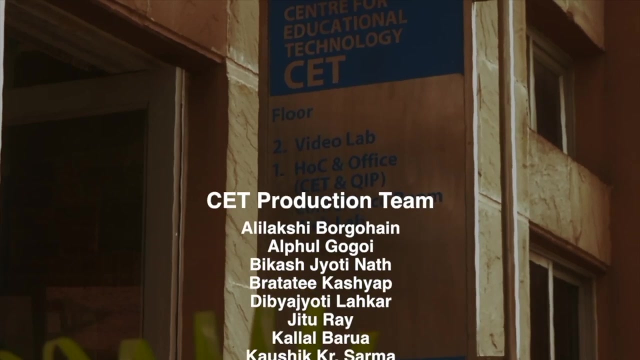 calculation also using this Janicki diagram. so this is, we can say this one Janicki diagram. So thank you this. in the next class, actually, we will be discussing about the effect of temperature on the liquid-liquid equilibrium. Thank you. 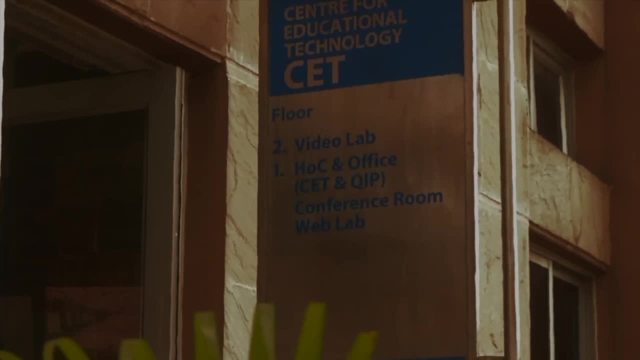 . . . .